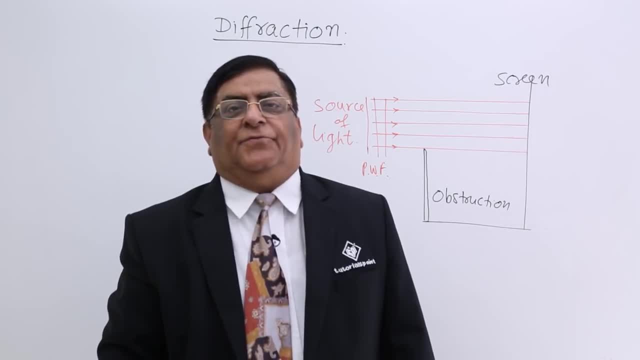 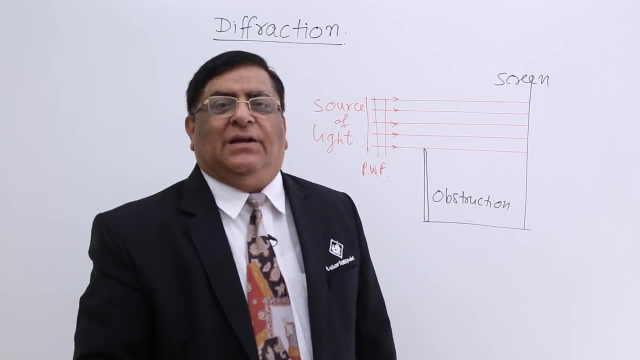 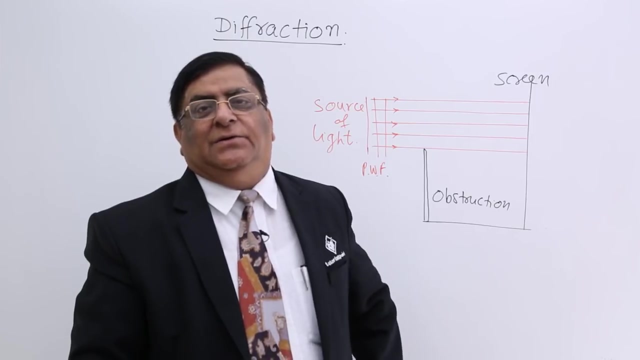 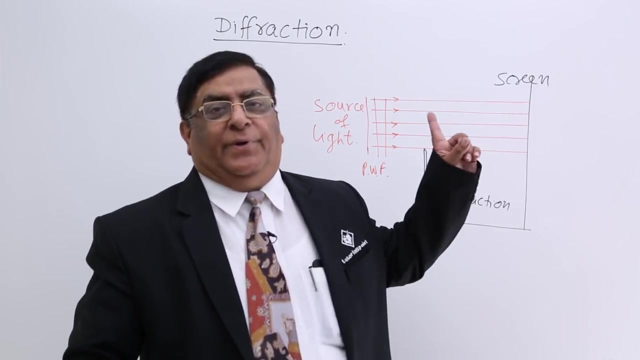 Today we will study a new phenomena: diffraction- Diffraction of light, And it tells us that light do not travel in a straight line. It was a very challenging statement- The light do not travel in a straight line- But we will show it in this phenomena that is diffraction. 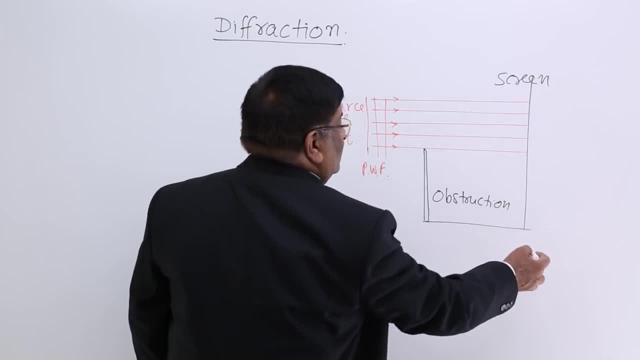 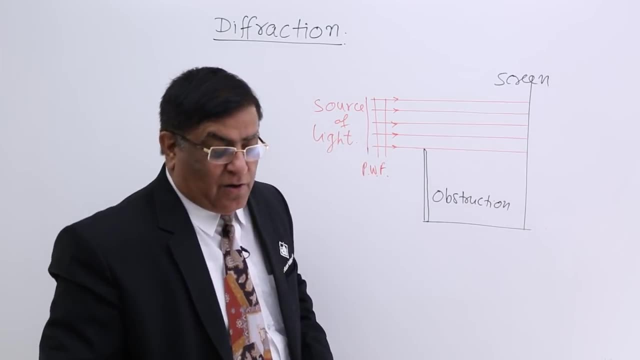 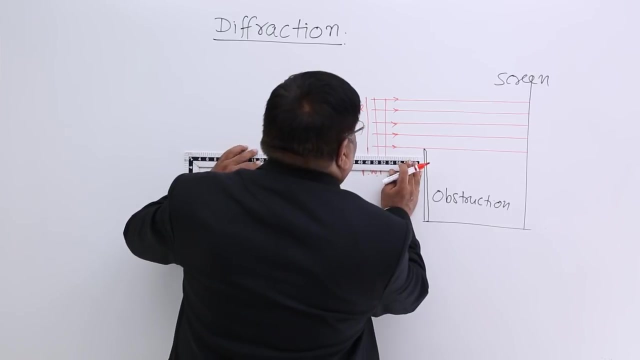 See, here there is a screen. We have put an obstruction here And we put it in the sun or in any such place where there is a light incident in this particular direction. And when you see the light is here, then on the screen there will be shadow. 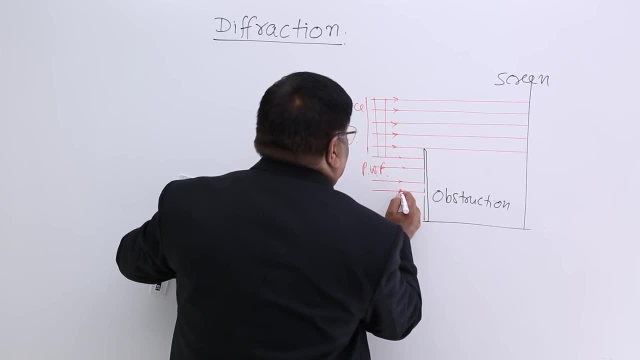 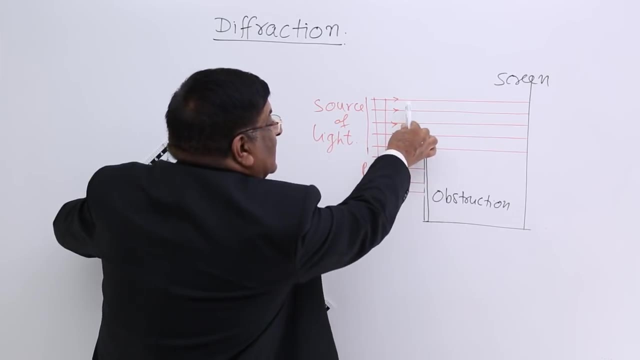 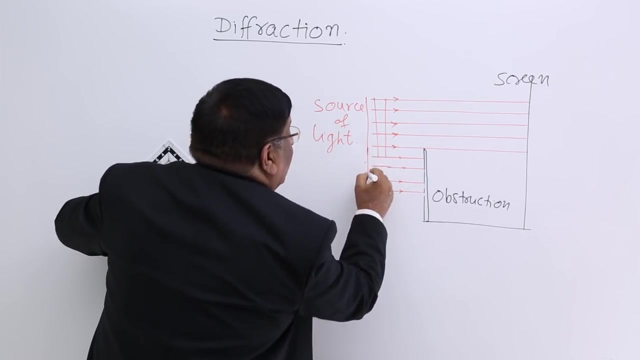 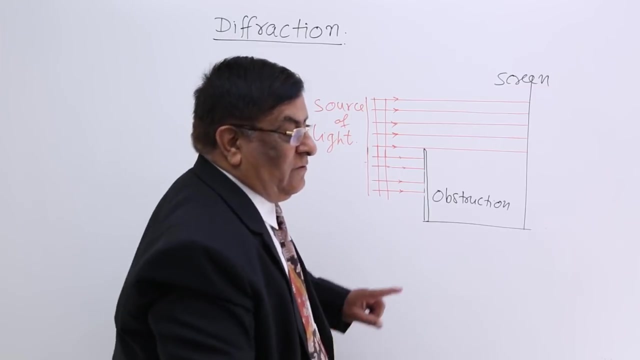 Okay, this much is sufficient. These are the lights. So this light is blocked by the obstruction. This light is allowed from the source, And we have these plane wave fronts. These wave fronts are moving in this direction. So what do we see on the screen? 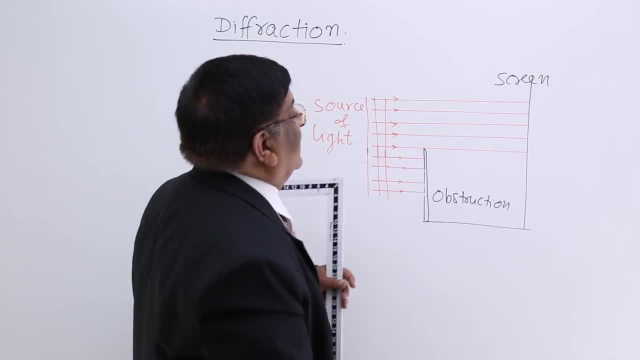 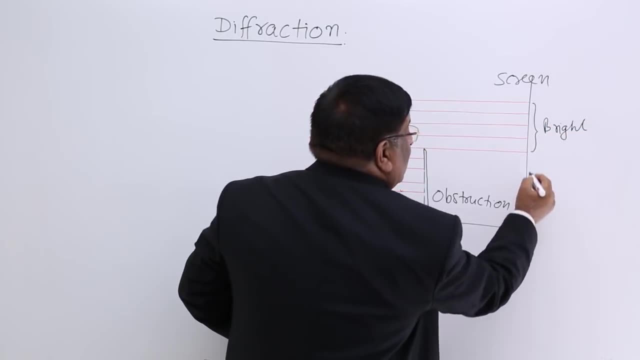 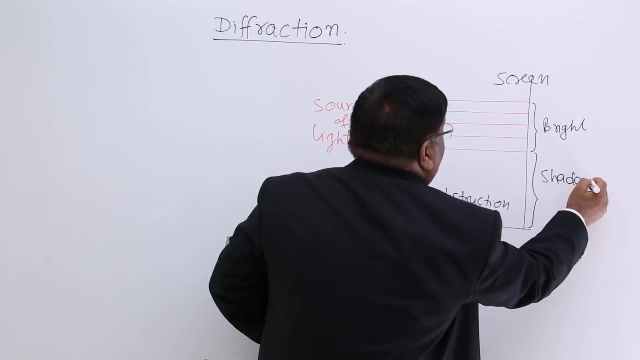 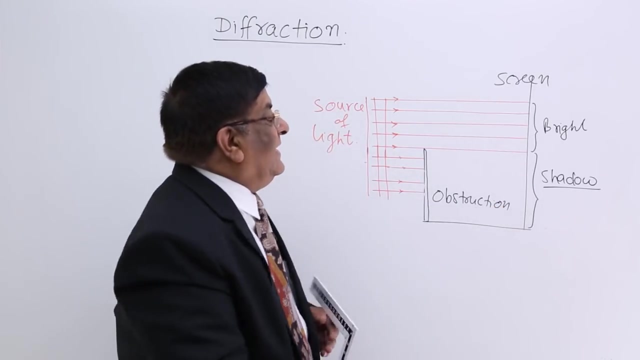 On the screen. we are supposed to see this area as bright area And this area as dark area. And this dark area we have a word to describe. We call it shadow. So there will be shadow of the obstruction on the screen. And where will be that shadow Up to this much? 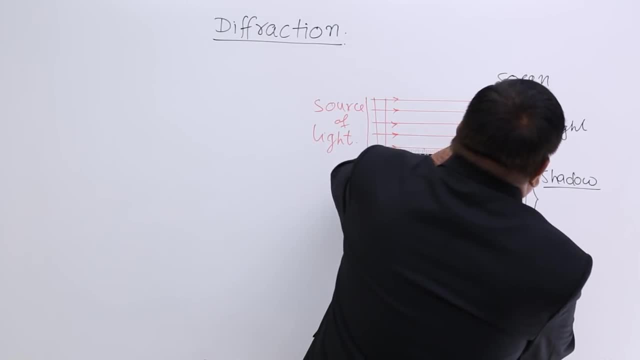 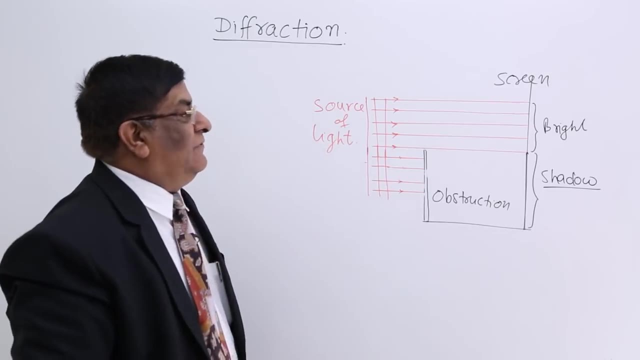 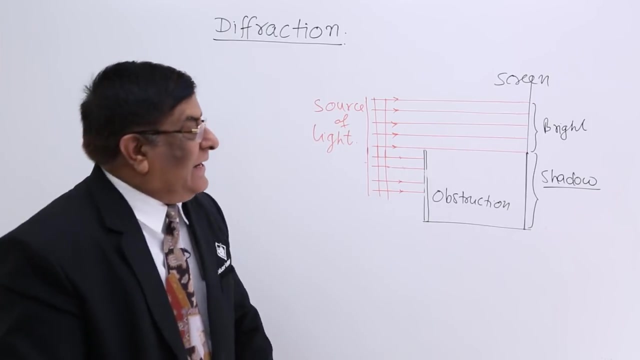 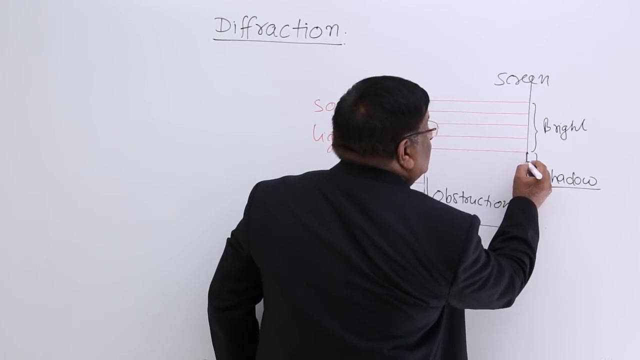 From this point. So this is the length of shadow. Okay, we can all make it by geometry. We know this When we do it practically in the lab, what we find: that this shadow is not up to this area And this shadow is only up to this much. 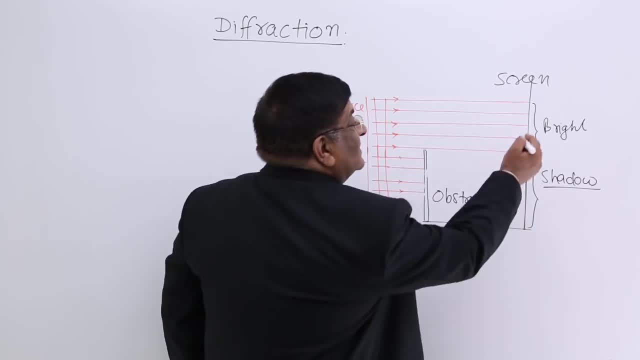 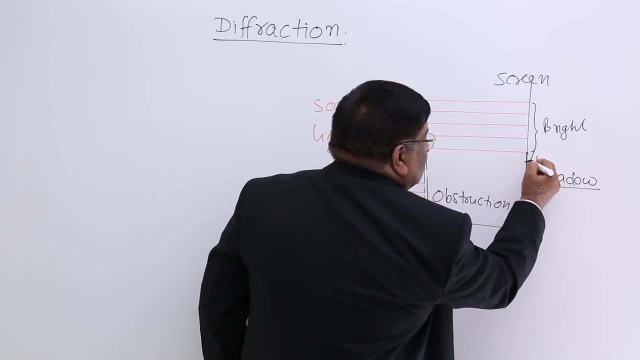 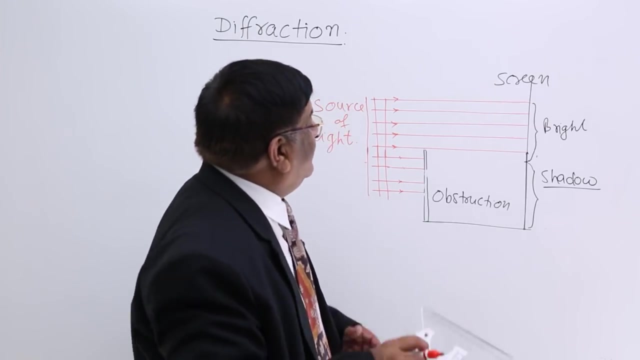 This much. What does that mean? That means this brightness is not up to this place. This brightness is up to this place. here It comes up to this much And the shadow reduced to this much. How the brightness is here? Our answer is: the brightness is here because some light has entered this area. 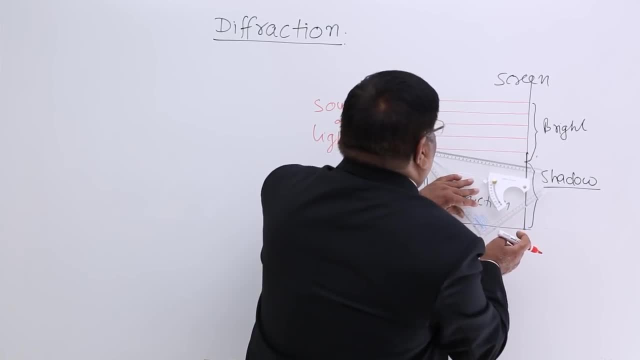 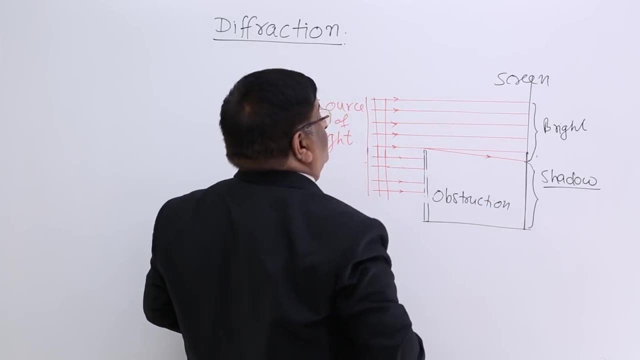 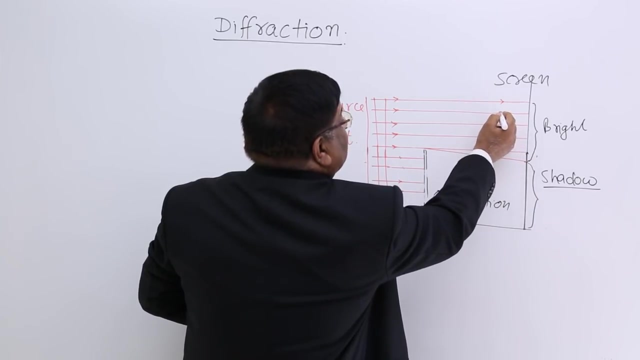 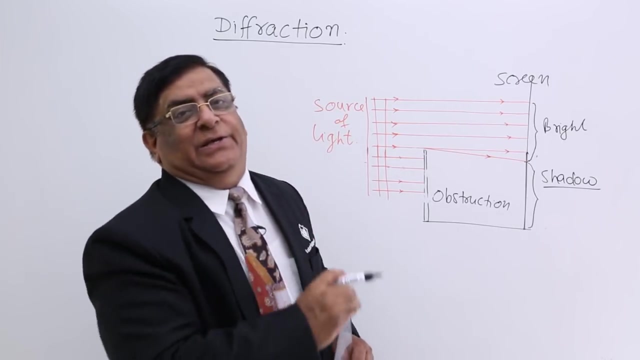 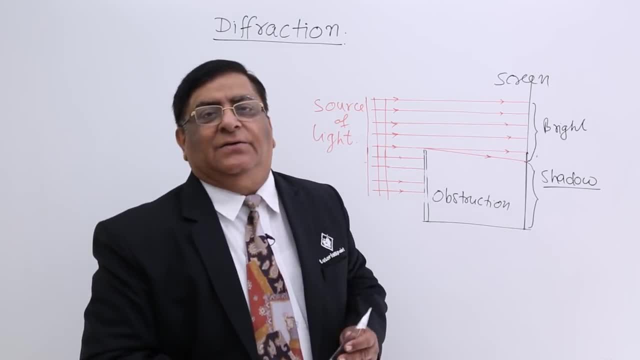 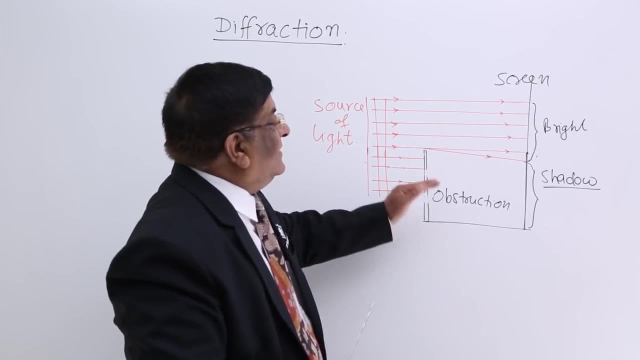 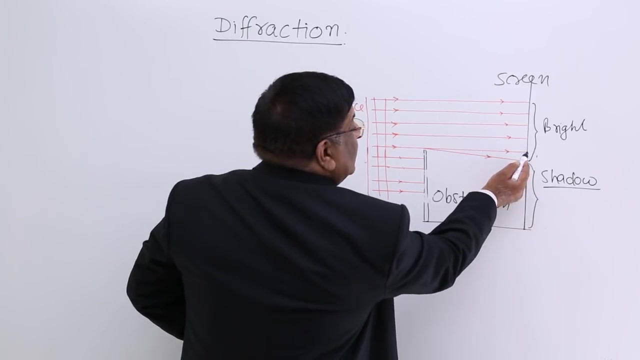 So when we see something, actually that becomes the phenomena of the nature. So what is phenomena of the nature? When the light cross an obstruction, then it bends and enter the shadow area. Geometrically the shadow should be up to this much, But practically it is only up to this much. 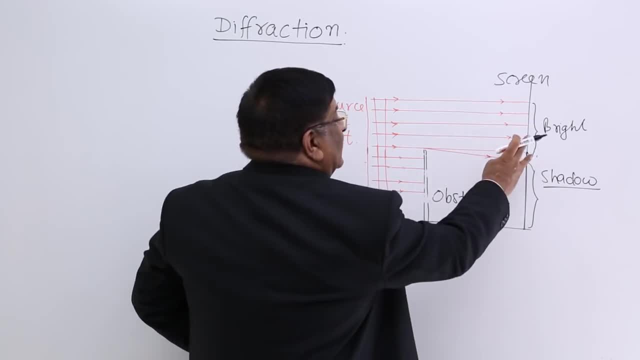 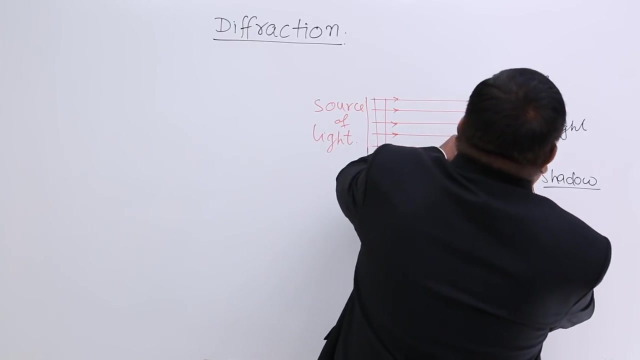 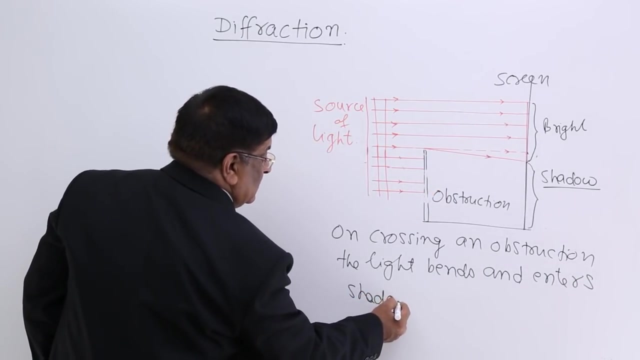 And because the light has entered the shadow area and we can say it is like this: Here also there is light, Here is light, Here is light And here there is also light. So this all area is now a bright area. On crossing an obstruction, the light bends and enters shadow area. 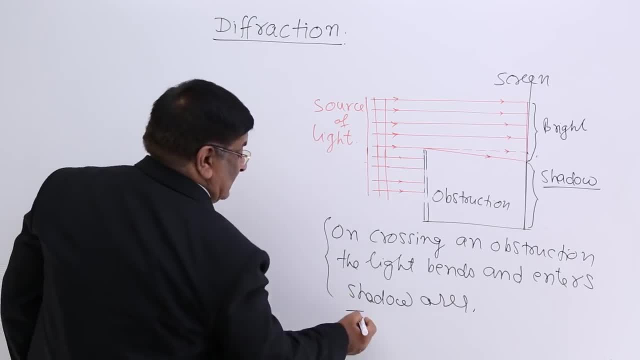 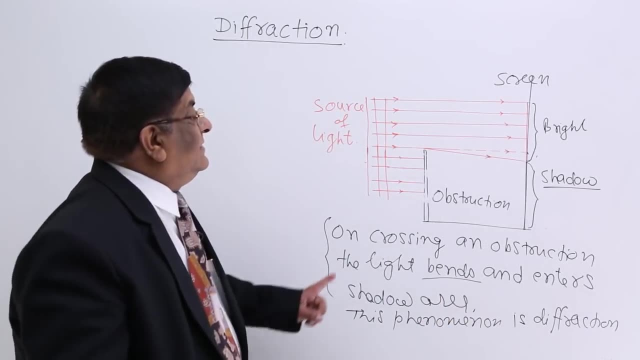 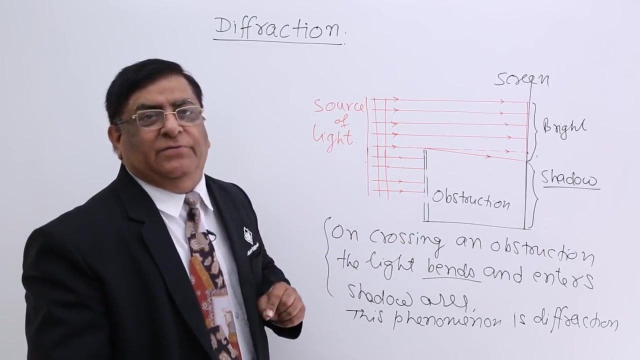 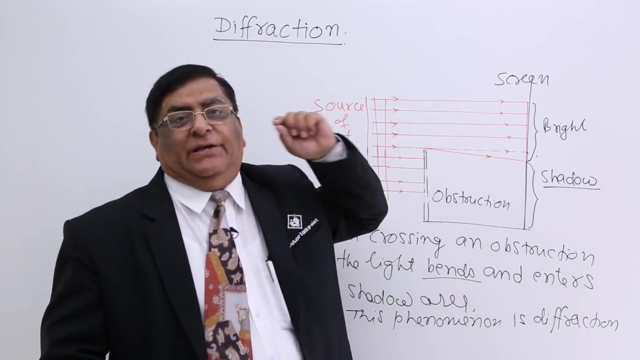 This phenomena is diffraction. What phenomena? The phenomena of bending. And this is the phenomena in which bend take place. And this bending has a rule. We have observed that this bending is never towards the bright area, This bending is always towards the shadow area. Obstruction side. 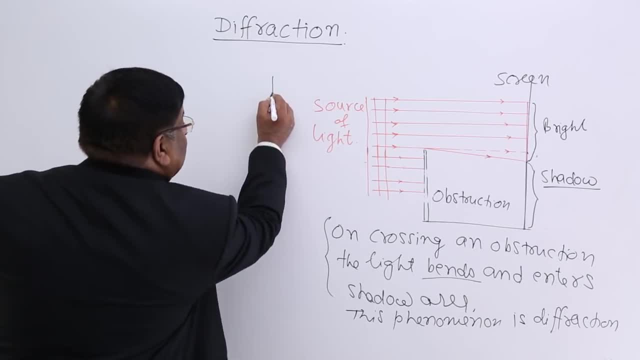 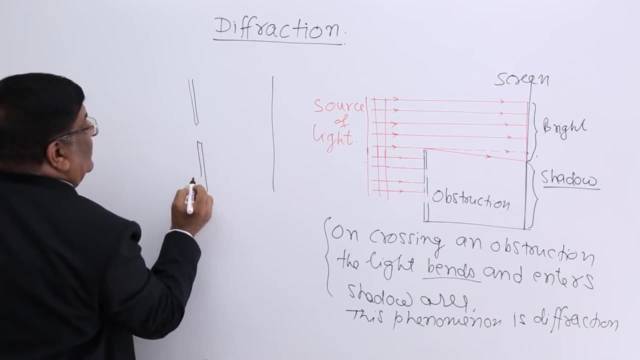 Okay, Now, if we have a screen here and we have two restrictions This way and the light is coming from here, What we find That here, this is the opening- say A: Here we find this area, the bright area, is not A. 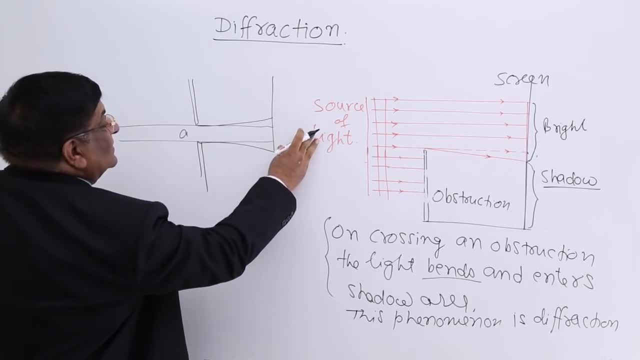 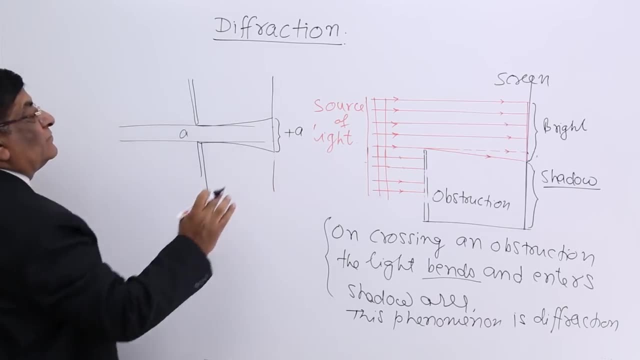 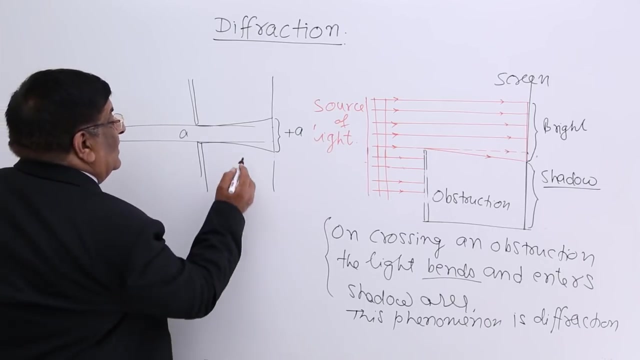 This bright area is this much. This is, This is plus A. So here the width is less, Here the width is more, And this can be explained only by the fact that light has bent in the shadow area of this And the light has bent into shadow area of this. 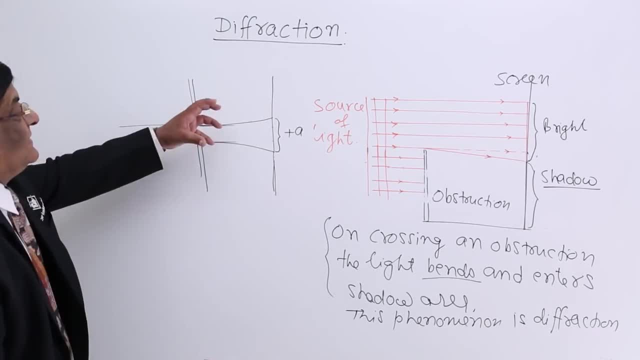 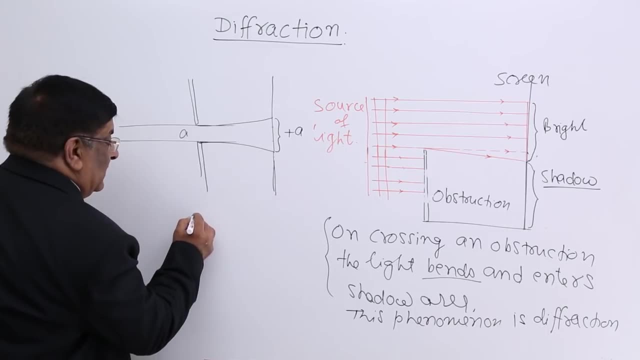 That is why this width is more, If the same thing we see for a circular opening. When there is a circular opening here, the light is coming from this side And here is the screen. We find A circle here Which is larger than this. 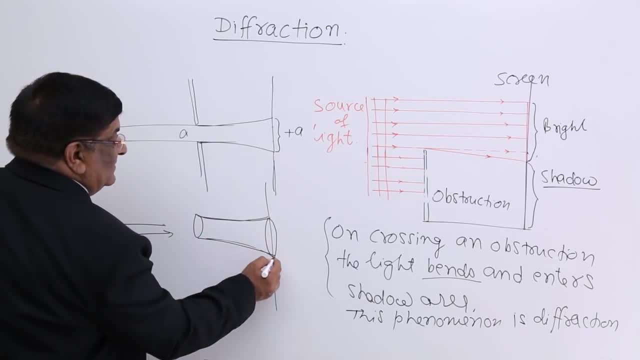 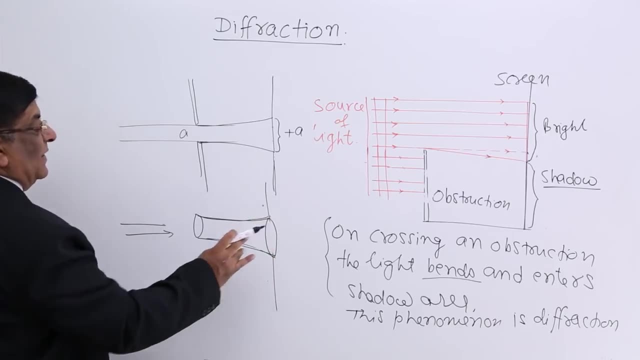 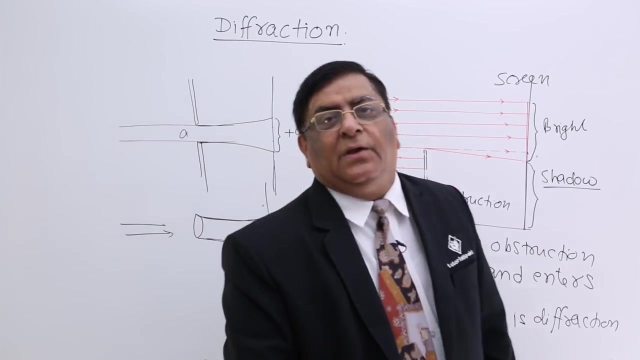 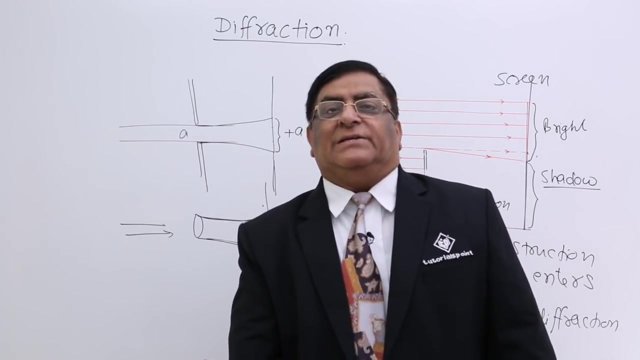 And that indicates the light has bent. Bent towards what Shadow area? So the bright area, circle area has become larger. All this is phenomena of diffraction. So this is diffraction. Now why it takes place? The answer is it takes place because of the nature of the light is a wave nature. 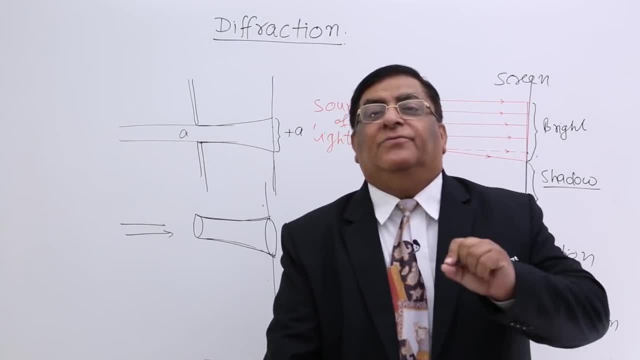 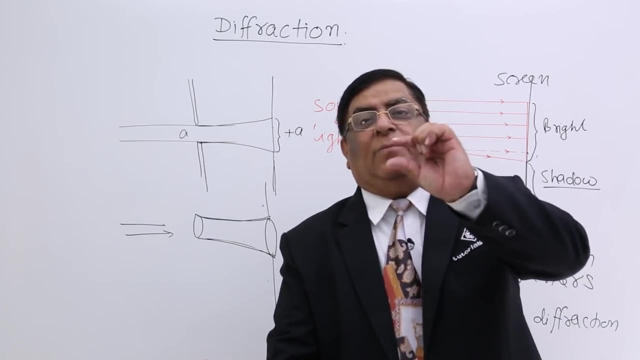 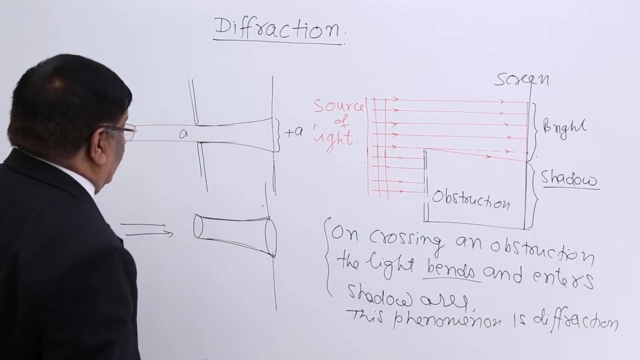 Because it moves in the form of waves. And we can explain that when it moves in the form of waves, then this opening will become larger. Now how to explain that this opening will become larger. You see, from this point to this point, there is no dark point here. 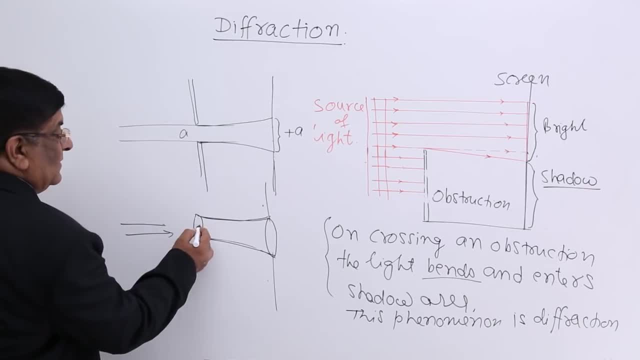 In this opening. all are bright Here again here. this is the dark point, And then it is all dark point. This is the first dark point. After that, all the dark points On this side. this is the first dark point. 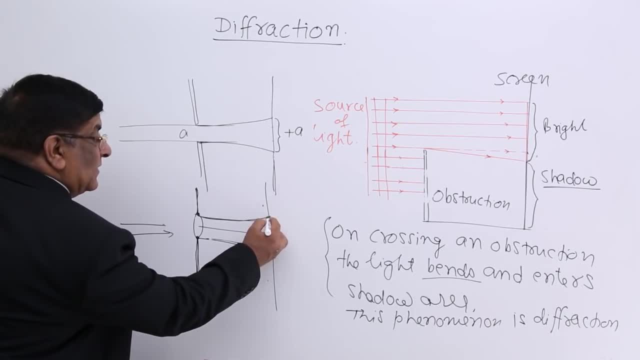 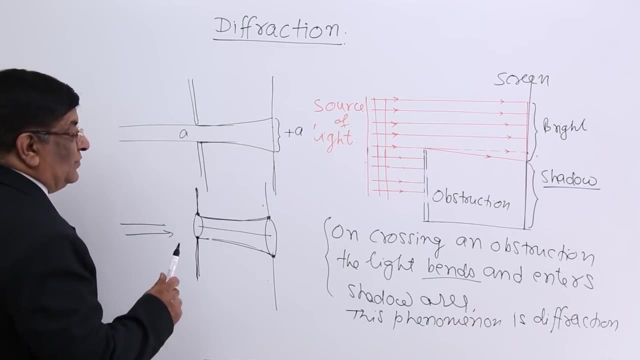 Then all dark points. Now here, this is the first dark point, And this is the first dark point. If we are able to prove that, due to wave nature, the first dark here has a longer distance than the first dark here, Then what will you see? 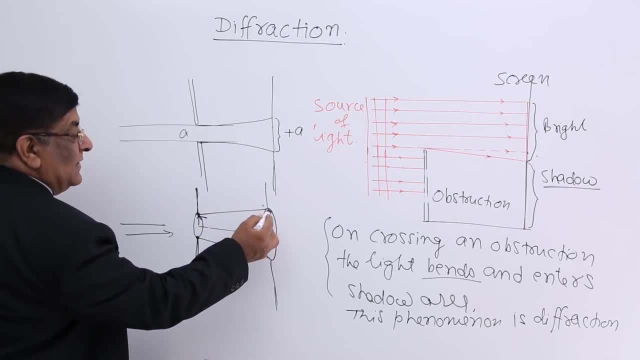 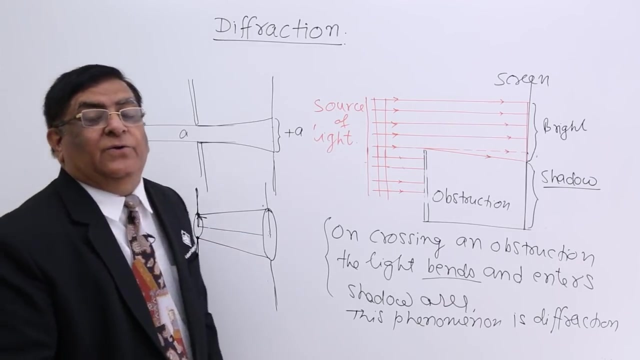 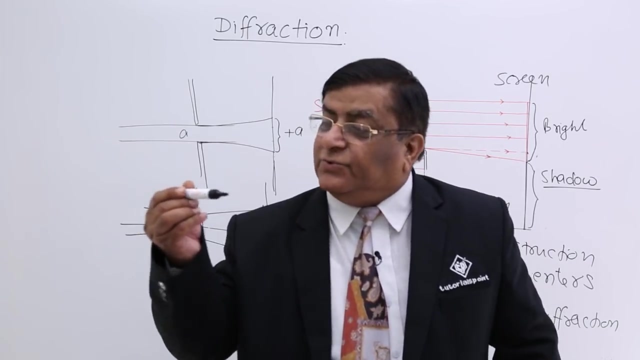 If this distance is larger than this distance, then what does it prove? It proves that the light has spread. The light has spread through the opening. And who is doing the spreading? Answer: a wave can spread, But something which is going straight will not spread. 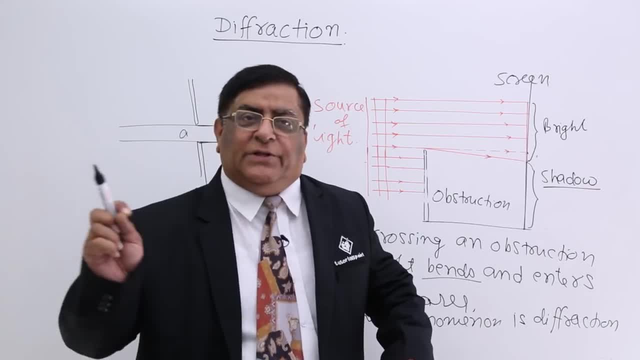 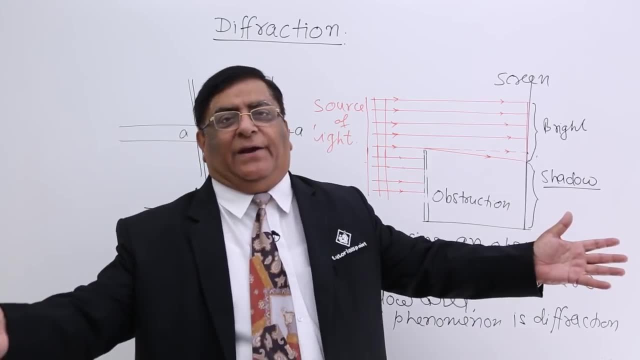 Like you fill up water in this room, open the door. the water will go out. Will it go in a line or will it spread? The answer is it will spread And water moves in waves. So it is the same nature with the light. 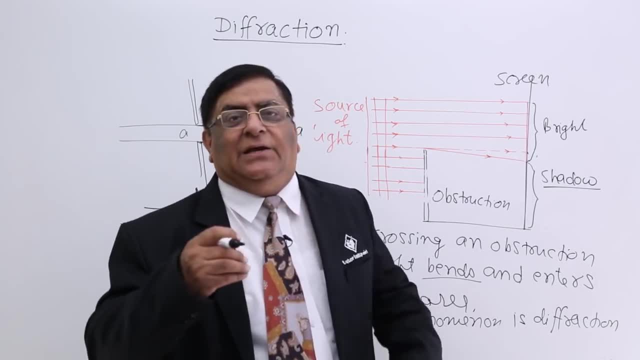 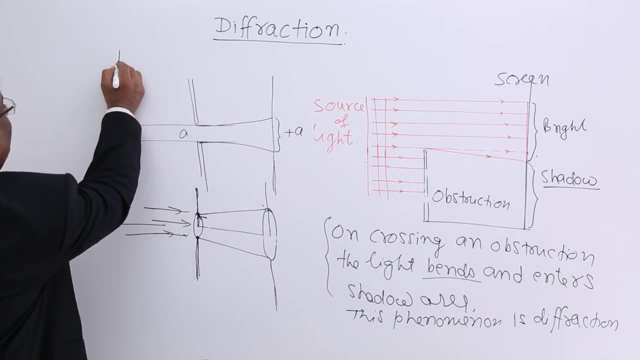 Whenever the light finds an opening, it does not move in a straight line, It just goes out and spreads. And that is what Huygens said: that if there is an opening like this and this point becomes a secondary source, The light will go here and it will start moving in this direction, this direction in all the directions. 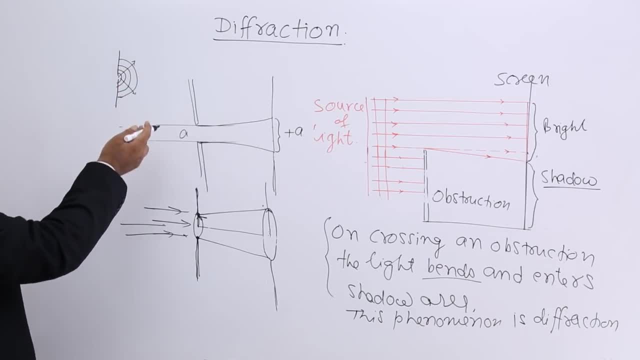 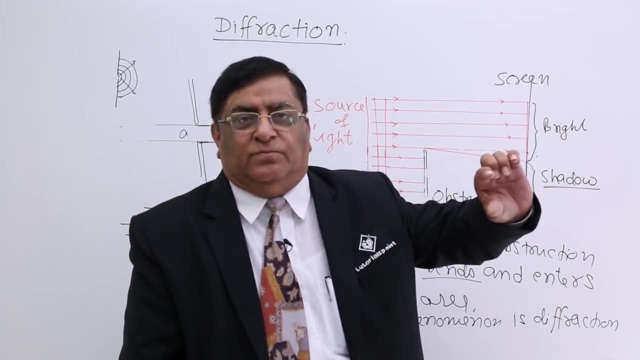 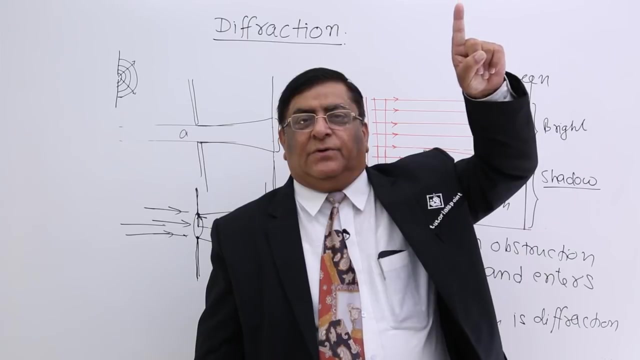 Just like waves of water. So the light will spread. And that is why, when we open a small window in the room, the light does not come straight. The whole room gets lighted up. We are able to see the roof, We are able to see the floor. 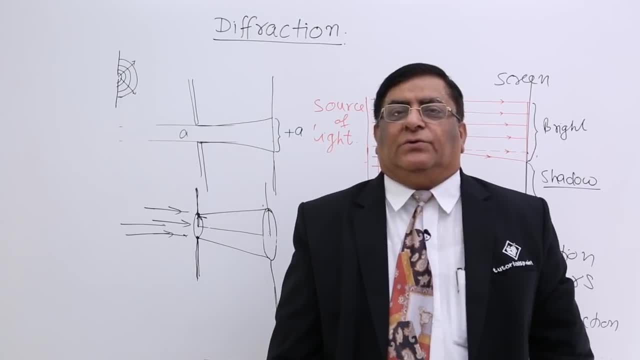 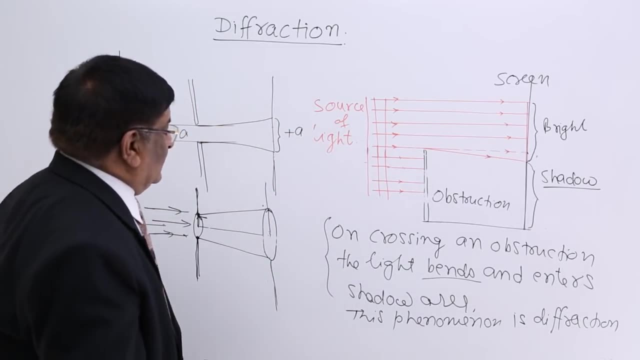 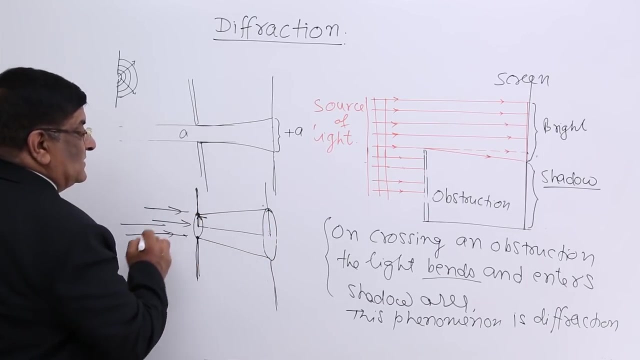 Why? Because the light has spread all over. So the basic nature of the light is spreading, not going straight, And that is diffraction. Now why this opening should appear large? Because here is the first dark and here is the first dark point. 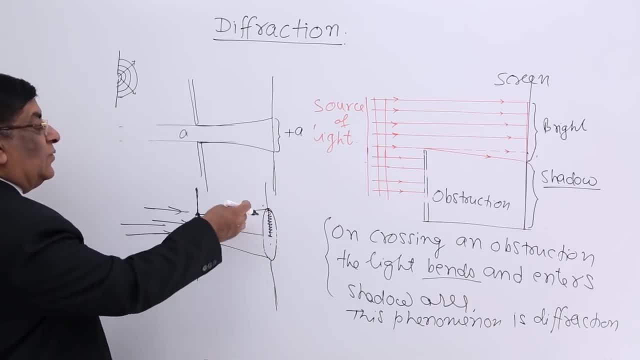 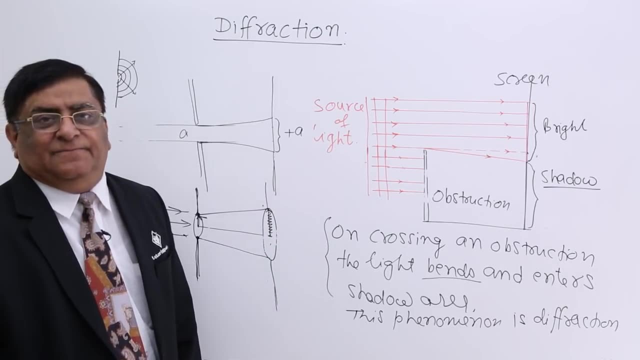 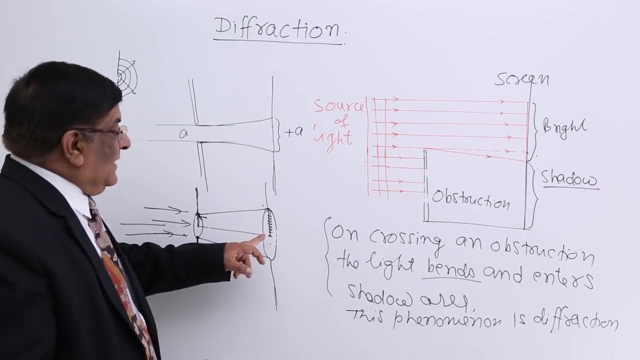 Up to this. there is no dark point. Can we prove it? How it happens? There are two things. One: we see it in the nature. It happens Everywhere it happens. Then we have to give the explanation That why it happens. 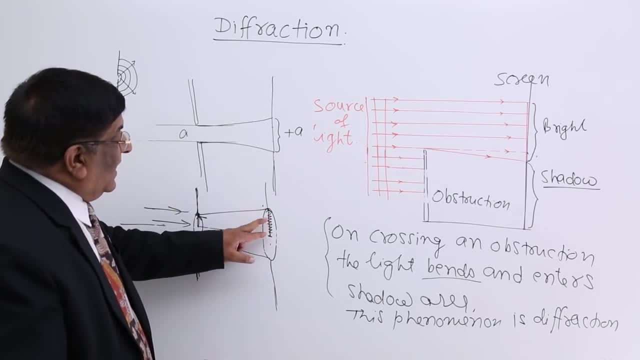 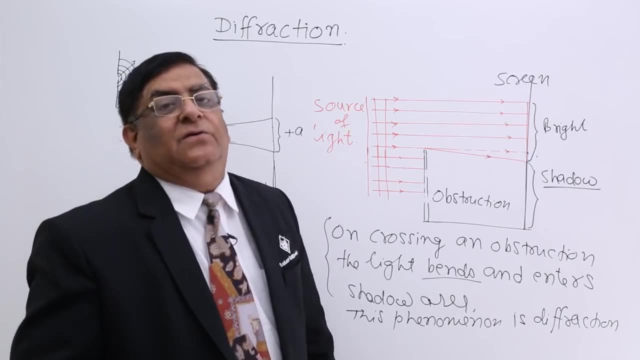 If it is dark, if it has got a certain height here. Here, the height of this dark point is larger than this and there is a bend like this And this we will explain. Here there is a cardboard and there is an opening AB. 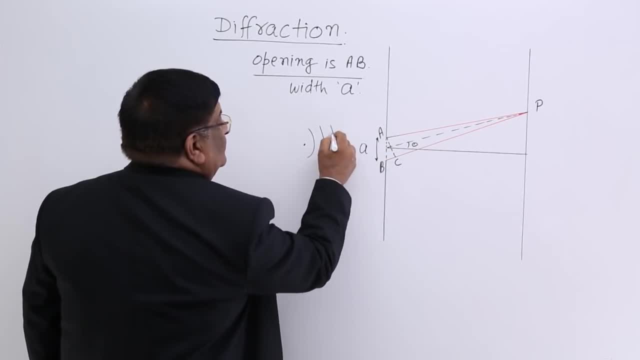 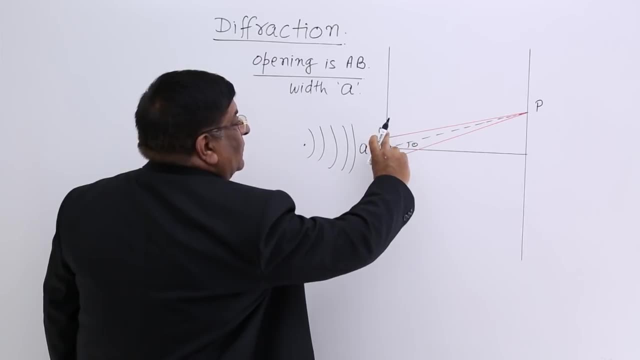 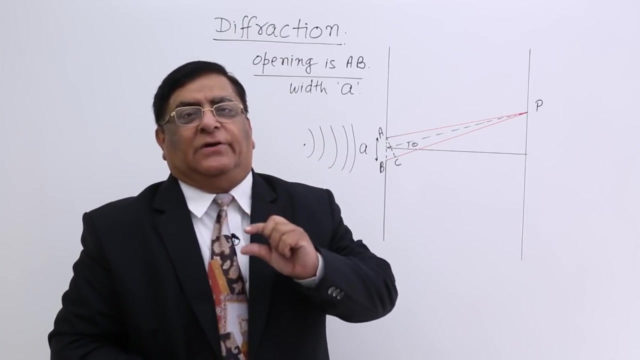 So the wave front from any given source. go and strike AB, Then this becomes a source of light for this area. This is a very small opening. Just for the sake of calculation, I have made it a bit wider. So what is the width of the opening? 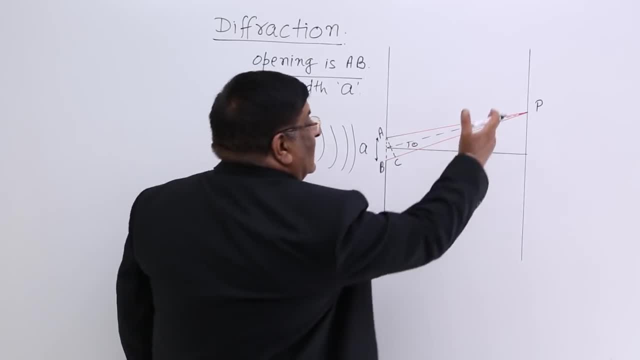 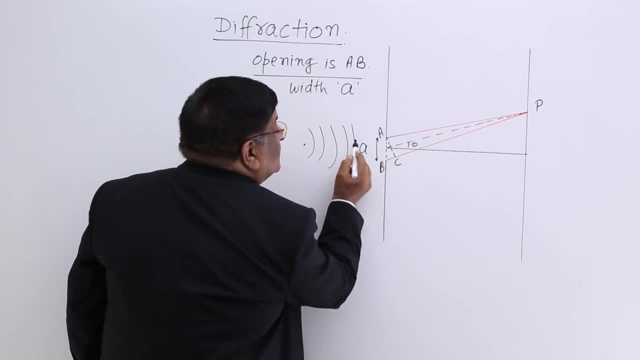 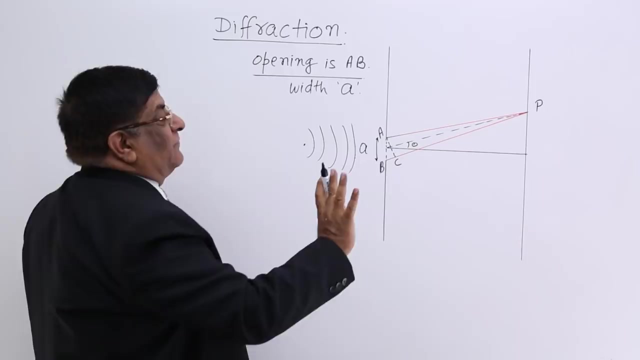 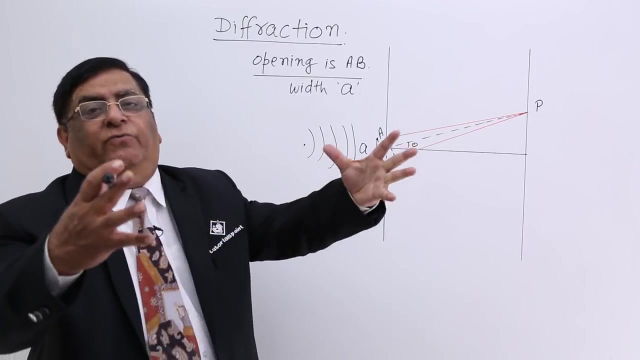 Opening width is A. Here is a screen, and this is a point. Now, in this opening, there will be so many points of the wave front which is striking this place. All the points will become source of light, according to Heisen's principle, and will start radiating their own waves. 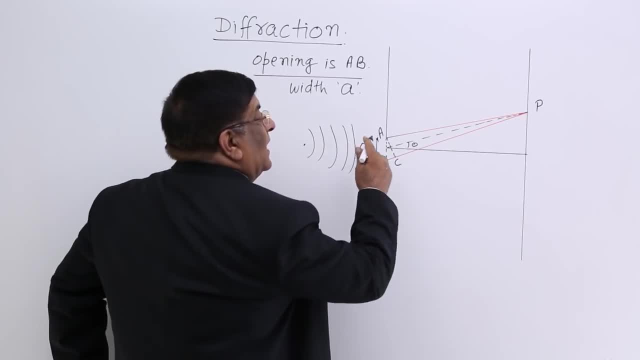 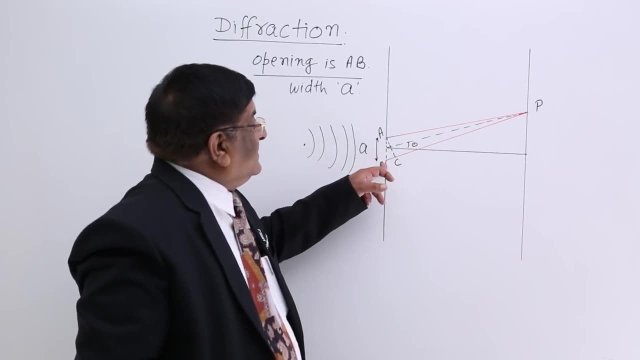 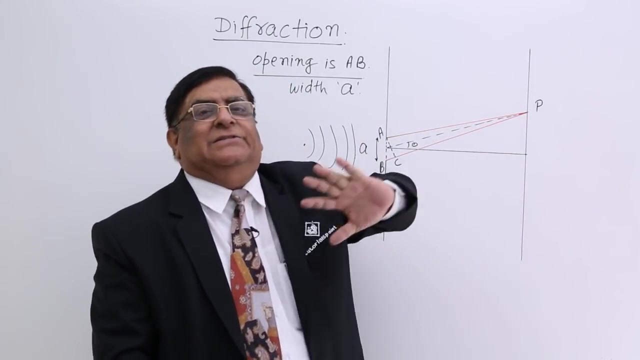 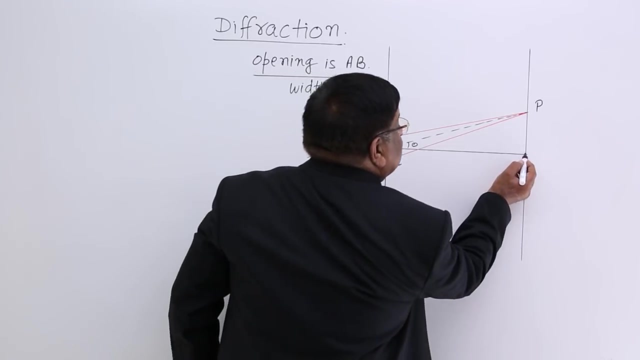 So point A and point B: both are radiating out, transmitting out their own waves, And all the points inside are making their own waves, And all the waves are moving towards this screen and the screen gets lighted up. Now, out of this we see that this is a very bright point, because all the waves reach here at the same phase. 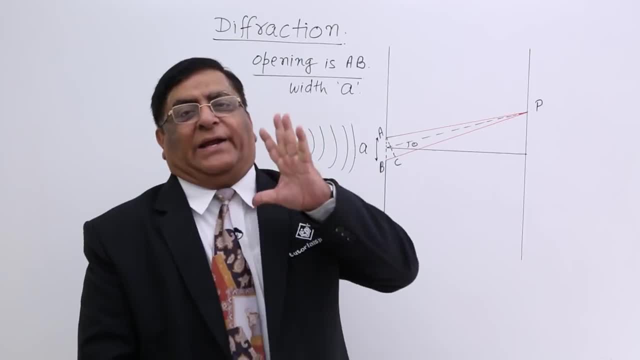 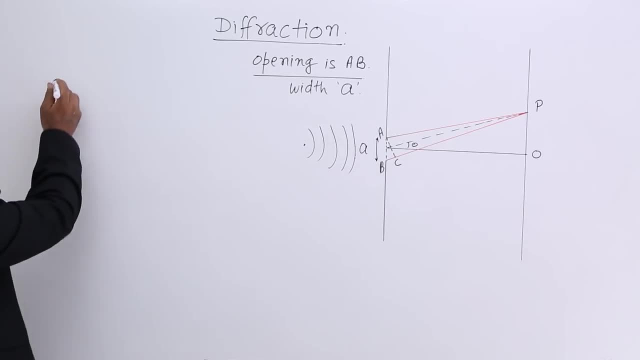 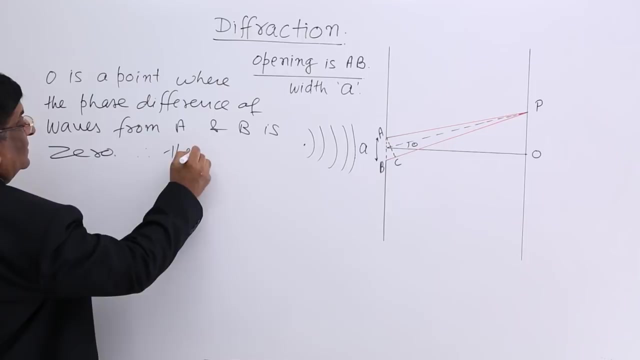 And when the phase difference is zero, the point becomes bright. So we give it a name, O, and write the description here: O is a point. The phase difference of waves from A and B is zero. Therefore there is constructive superposition. 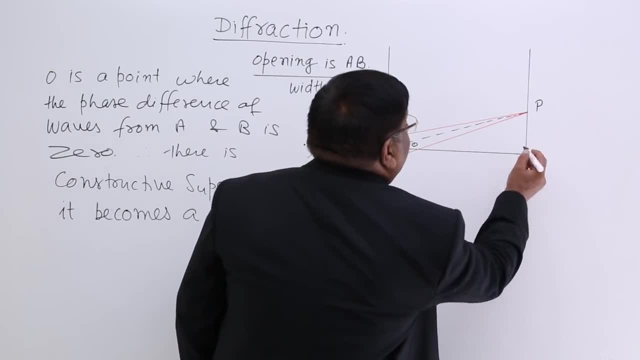 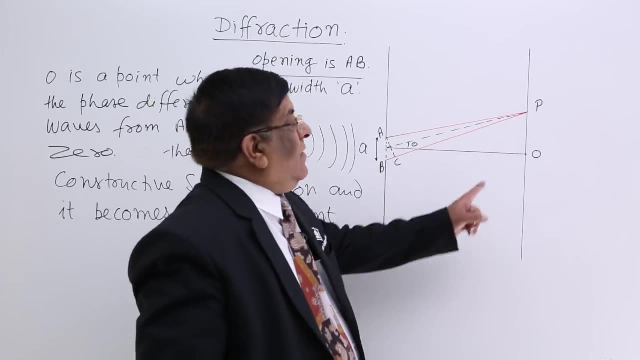 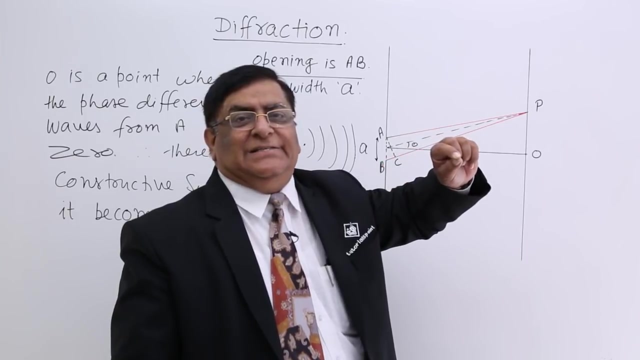 It becomes a bright point, or I should say the brightest point on the screen. So this O becomes the brightest point. Now, when we go on either side, we find the brightness decrease, decrease, decrease, decrease and a point comes where the brightness is minimum. 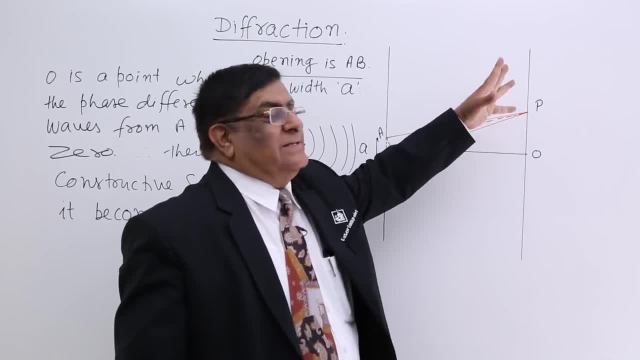 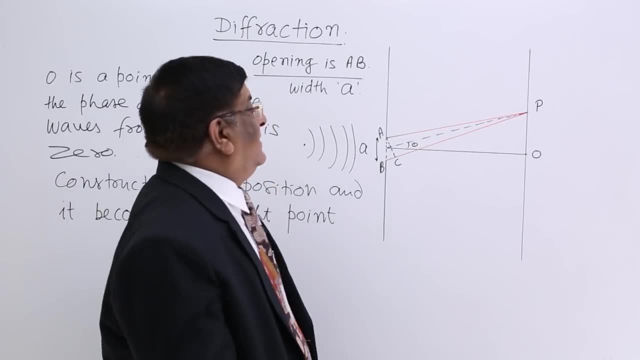 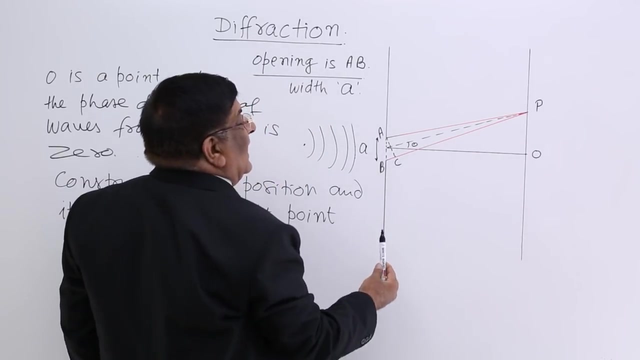 We call it dark point. So P is the dark point. If P is dark point, why? We find that the waves going from A has certain path length. Waves going from B have certain path length And there is a difference in the length. 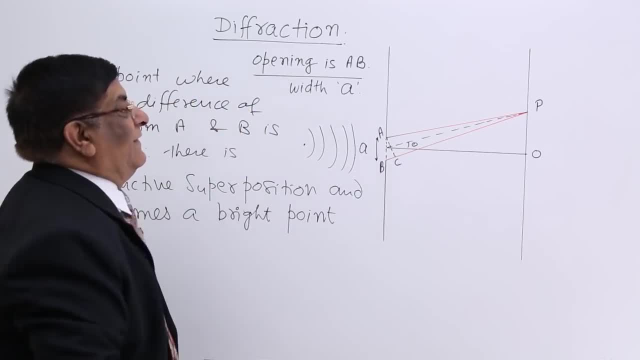 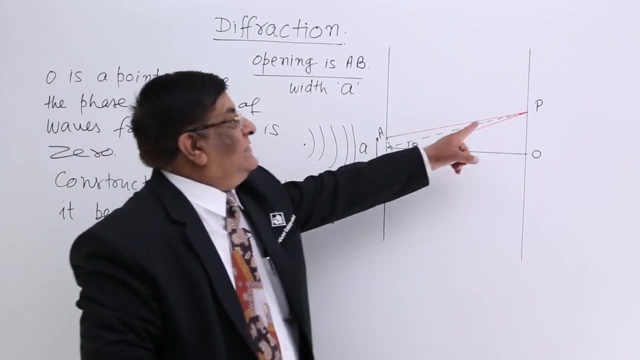 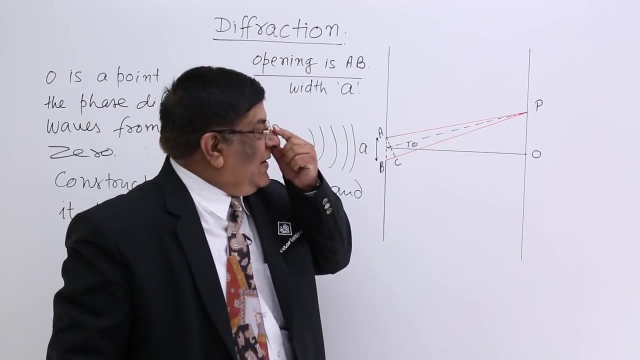 You are seeing the difference. BC is the difference in the length And this path difference when it is equal to 1 lambda, then we see point P is a dark point. When the path difference is 1 lambda, Number 1, could you understand why BC is the path difference? 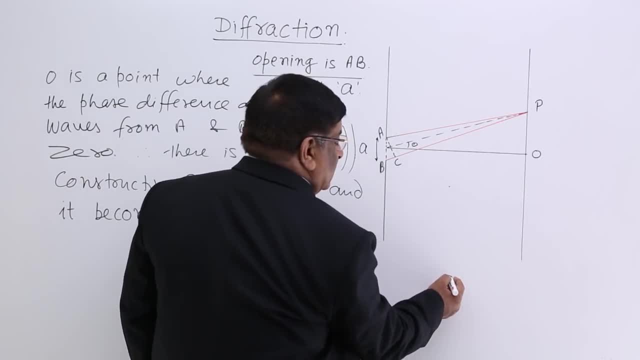 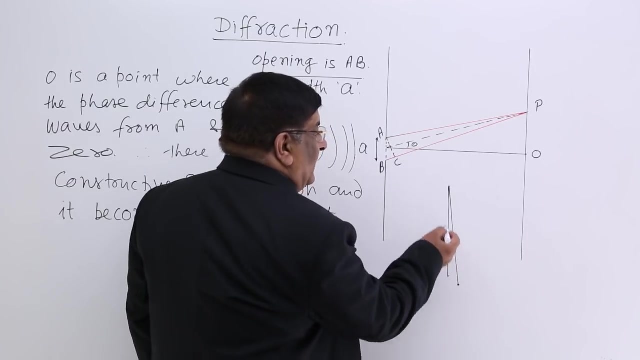 See, if this is a point and there are two sources here. This source, this is the length of the path, and this source, this is length of the path. Then what is the difference in the path? There are two methods. Either we measure the full path length and reduce, or minus this length from B. 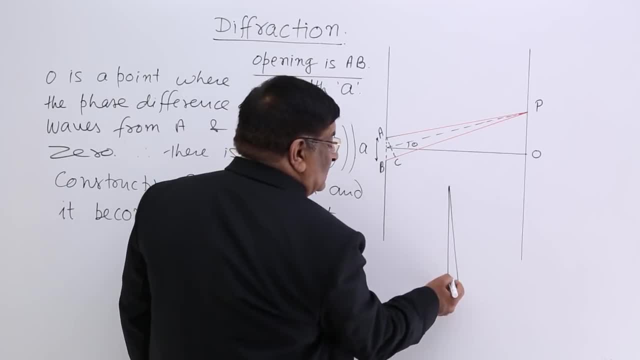 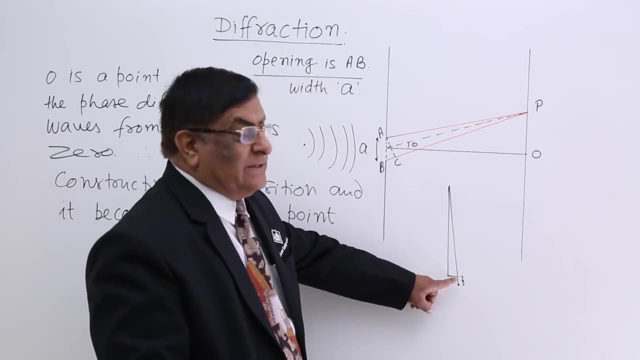 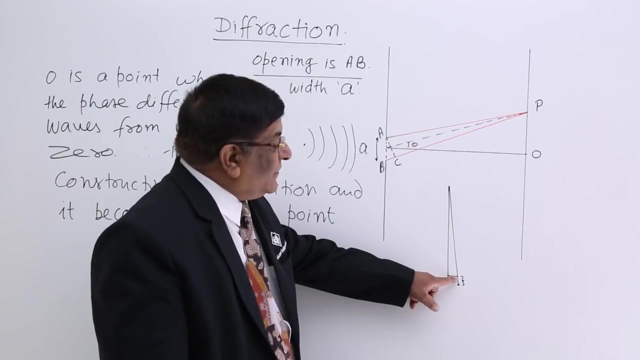 There is another method. If this angle is very small, draw a perpendicular here and measure this. This is the difference of path length, because these two are supposed to be almost equal. So this drawing a perpendicular gives us instantly, immediately, the difference of the path. 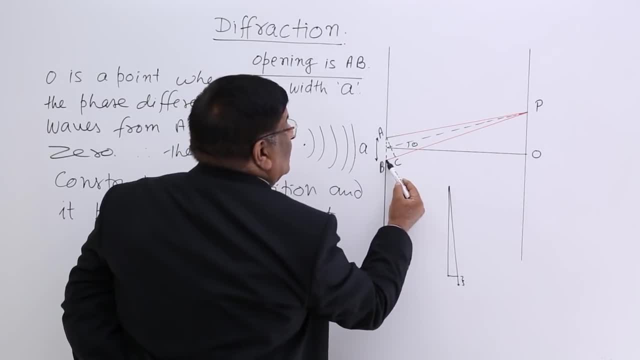 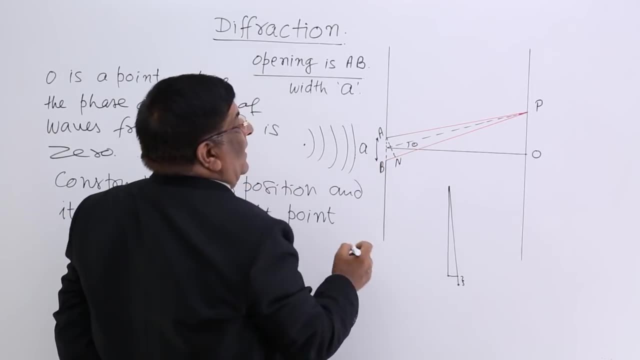 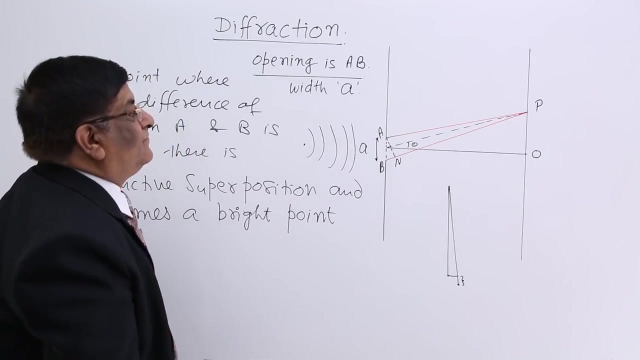 That is what I have done here. This is path length AP, This is path length BP, And if I draw a perpendicular here, then this AN normal BN become the path difference. Length of the path. length of the path. BN is path difference. 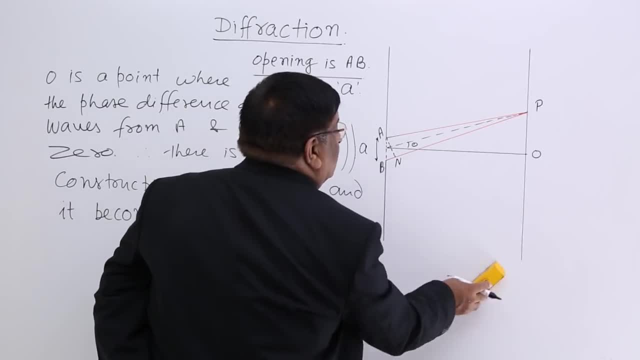 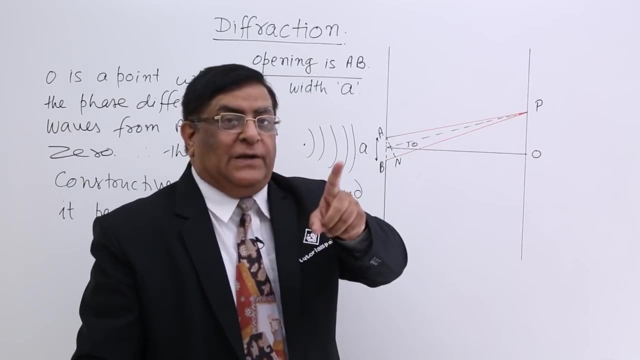 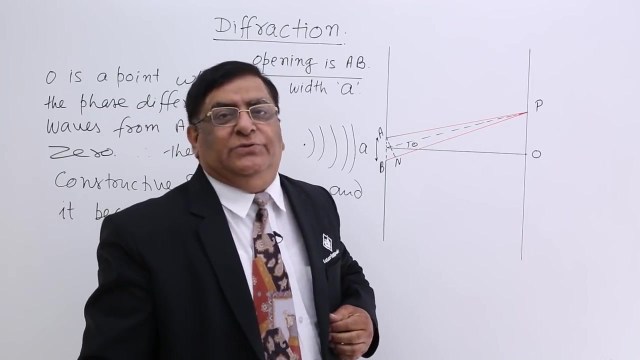 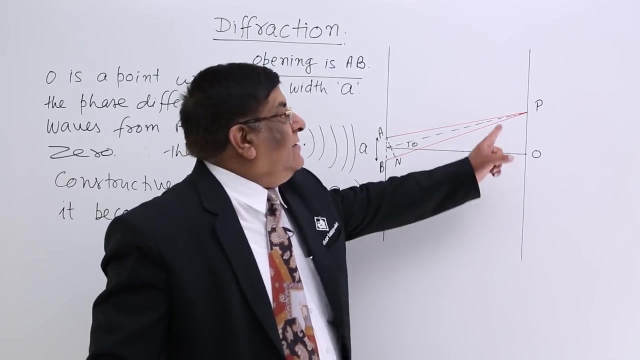 So if this path difference is equal to lambda, we have found that P is a dark point. If you recall, in interference pattern, what did we say In constructive and destructive superposition? what did we say? If the path length between two waves is lambda by 2, then the point of superposition is dark point. 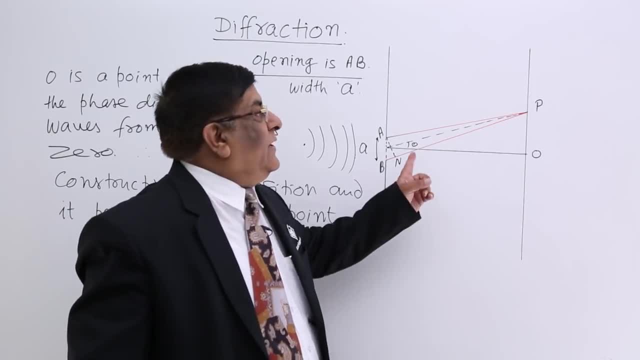 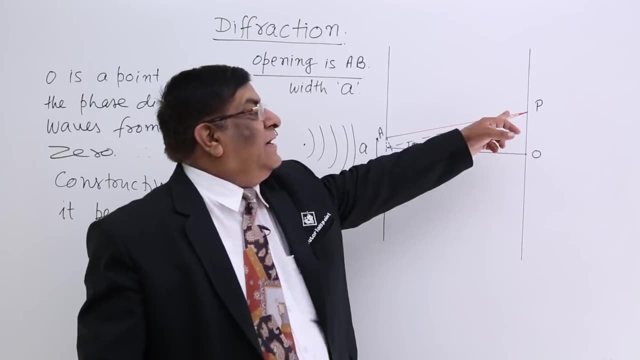 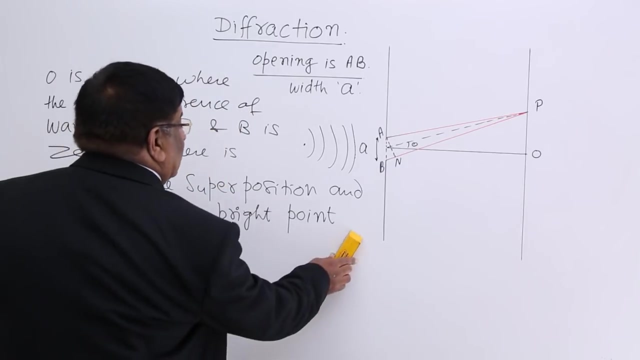 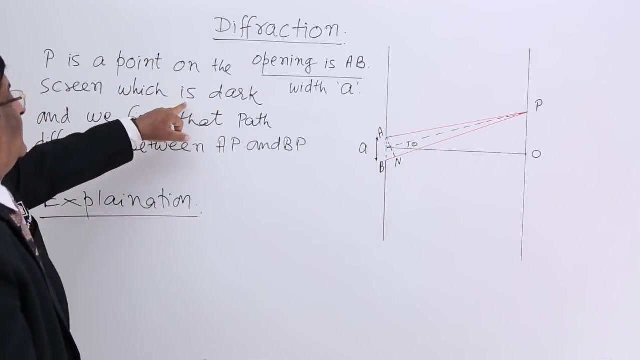 And if the path length is lambda, then that point is a bright point. But here what we find actually the path difference is lambda and P is a dark point. We will explain how it happens. First we write it down: P is a point on the screen, such that the path difference between AP and BP is lambda, and then it is a dark point. 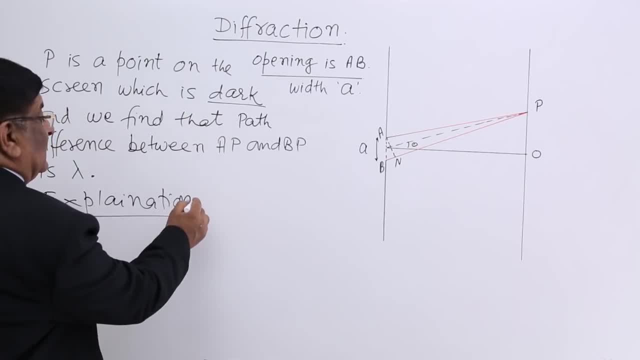 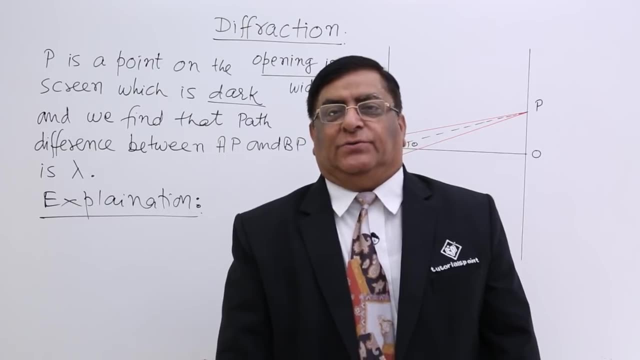 P is a dark point. What is the explanation for this? Because we understand in superposition, unless path difference is lambda by 2, the crest and trough will not be at the same place. it will not be dark. Okay, I show you. 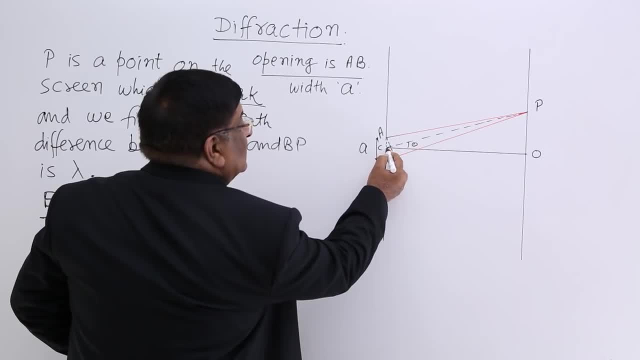 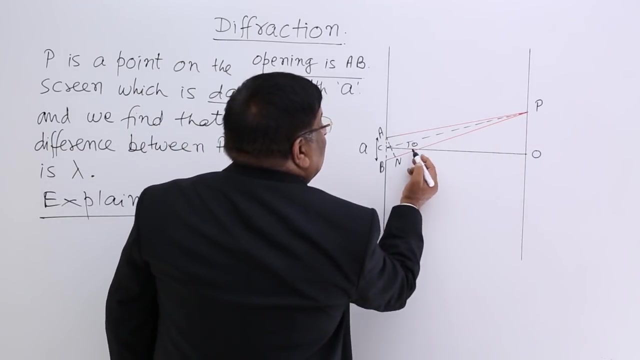 This point C is the centre point. If the path difference AP and BP, that is BN, Do we know how much is the BN? We can, very well, This P point has an elevation theta From this line it has an elevation theta. 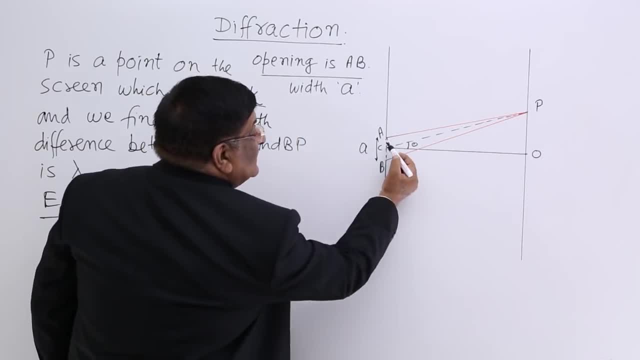 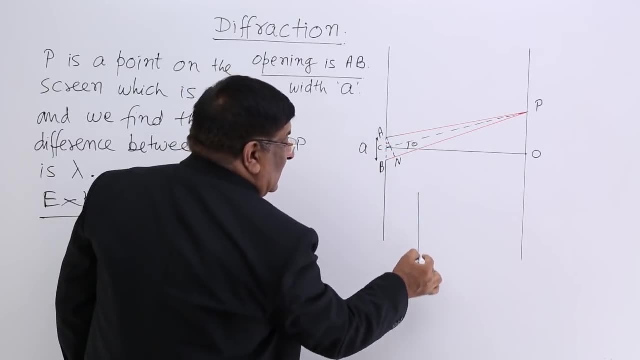 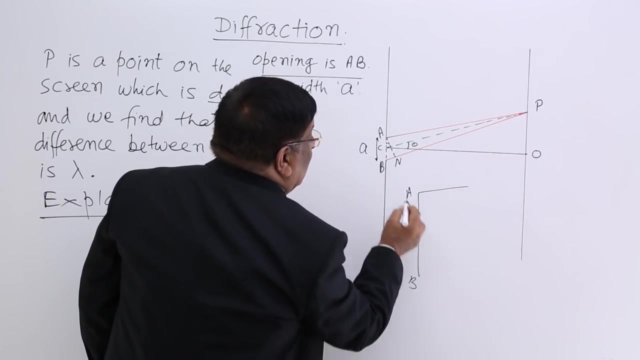 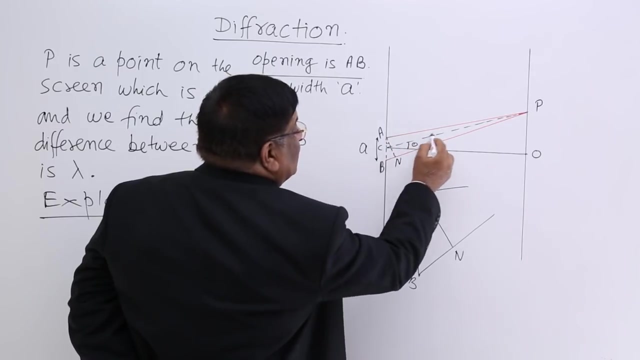 If this angle is theta, then this angle is also theta. I make this triangle here AB, AB, AP this direction and BP this direction. This is perpendicular on it, AN and this angle is theta. Why this angle is theta? Because this angle is theta. 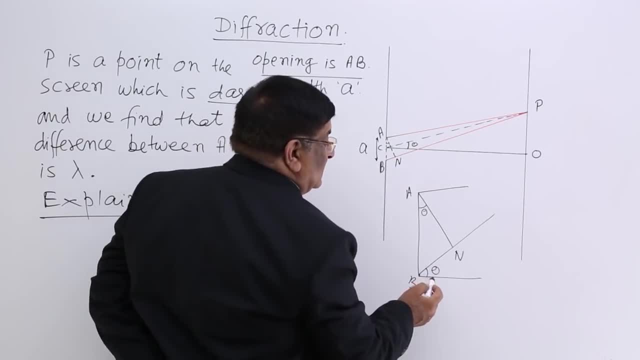 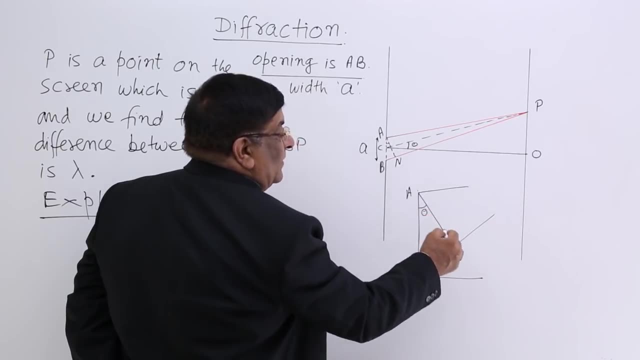 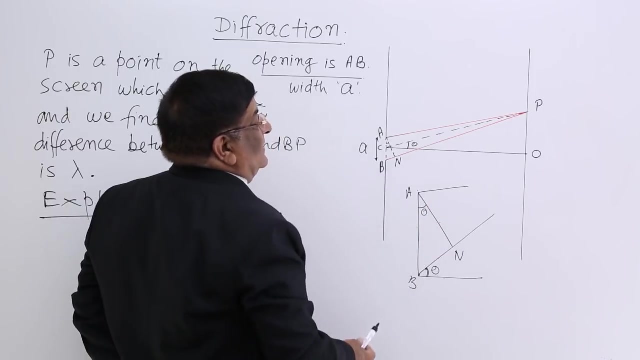 This angle is theta. If this is theta, then on this line, this is perpendicular. On this line, this is perpendicular. So if the angle between the two lines is theta, the angle between two perpendicular is also theta. See here. 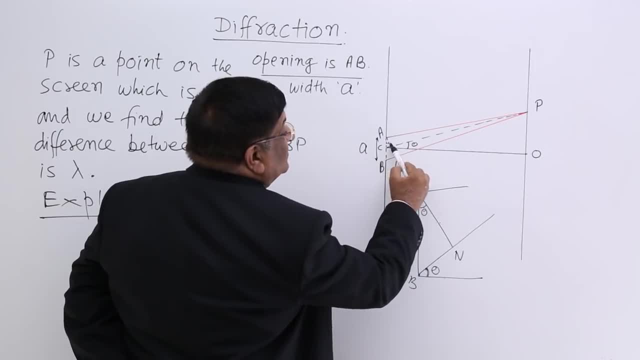 On this line. this is perpendicular On this line. this is perpendicular, So the angle between this line and this line is theta. Therefore, angle between their perpendicular is also theta, So this is theta. Now, this opening from A to B is A. 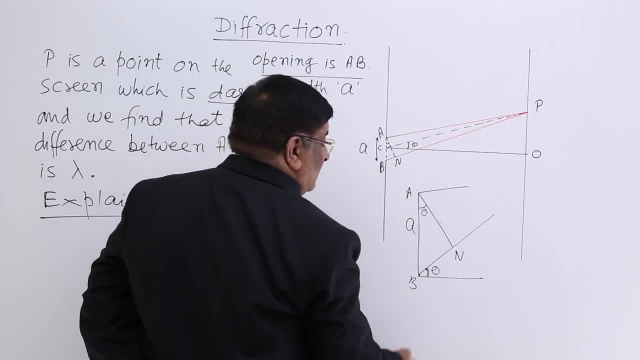 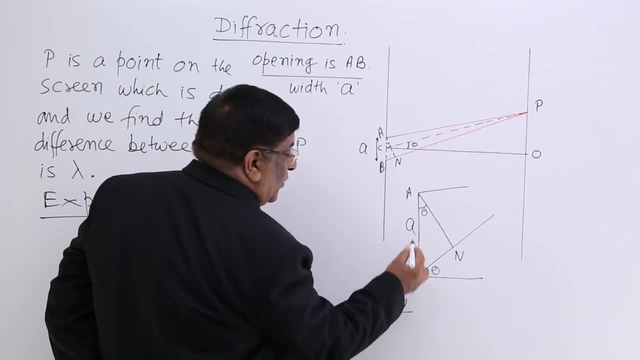 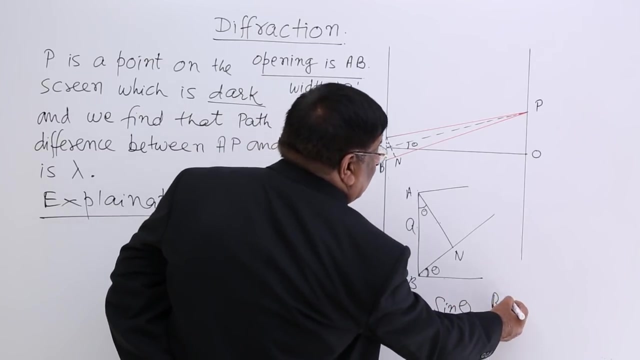 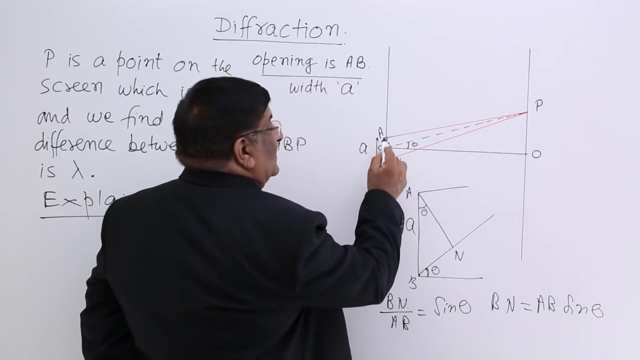 And what is the path difference? BN is the path difference BN. Now, in this triangle ABN, we have BN upon. AB is equal to sin theta. This gives us BN equal to AB sin theta, AB sin theta And AB has the size of opening A. 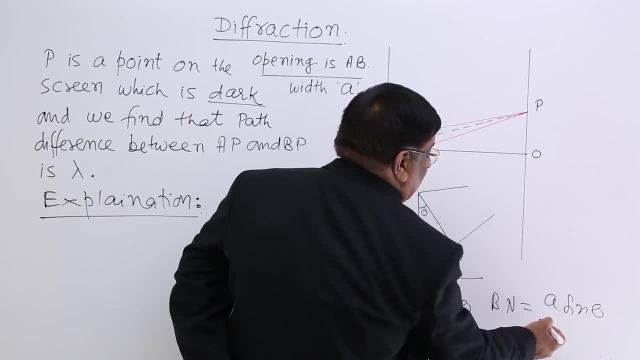 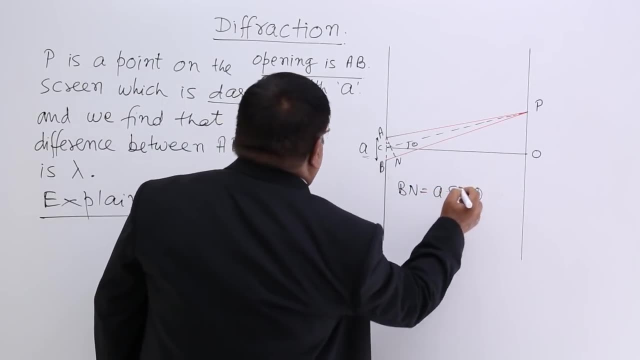 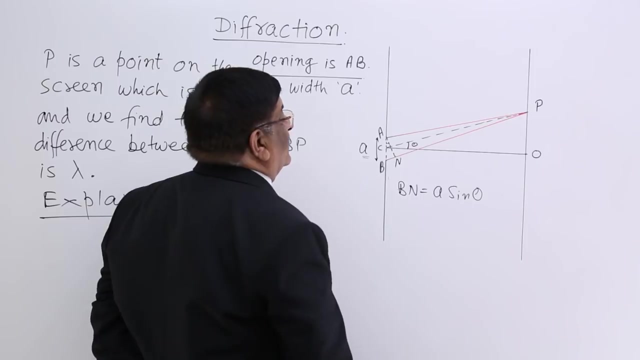 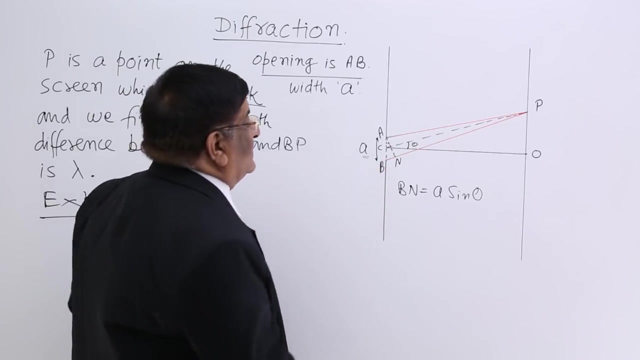 So we can write it: A sin theta, A sin theta. This is the path difference. BN is equal to A sin theta. That is the path difference. C is the centre point of this opening. Now the wave from A and the wave from B has path difference equal to lambda. 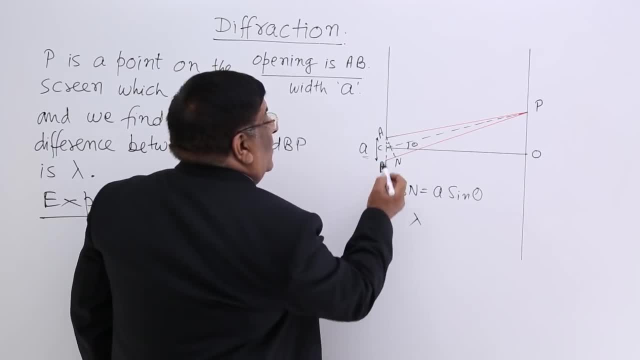 This is the centre point. Now, a point here and a point here. they also sending waves, And what should be the path difference between these two waves? Answer: the path difference between wave from this and wave from this is this much, which is lambda by 2.. 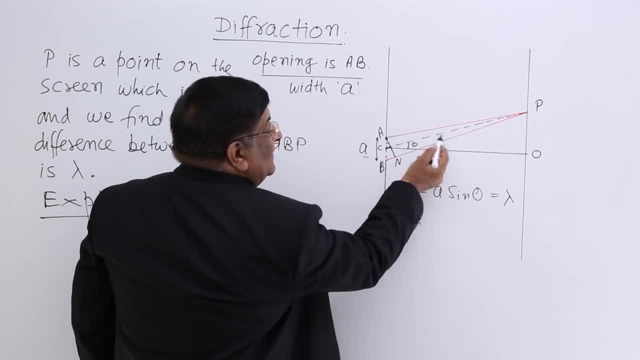 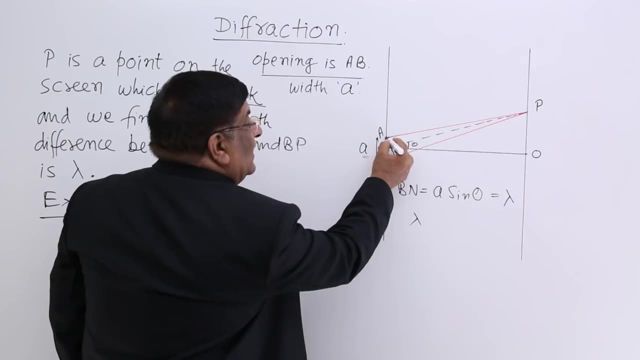 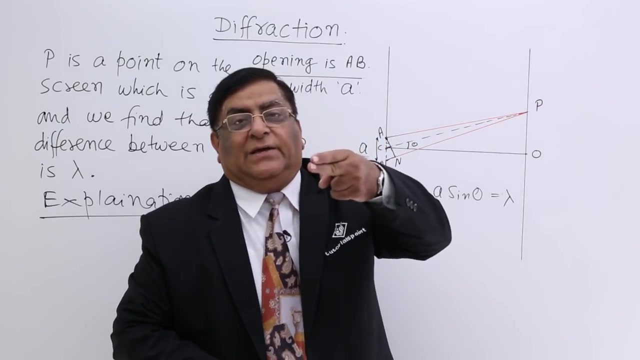 Because path difference between this and this is one lambda. So how much will be this Lambda by 2.. Now, a wave from A and one wave from C. they go here and at point P they superpose. When they superpose here, what is the difference between their path? 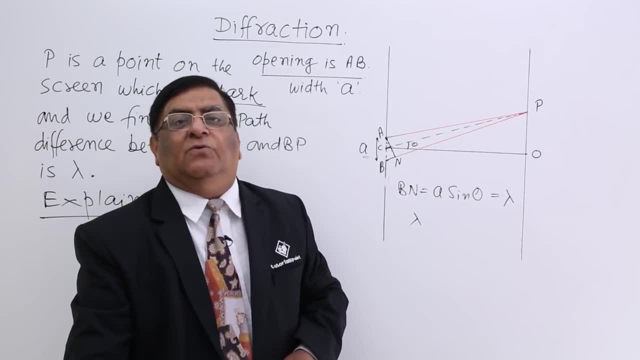 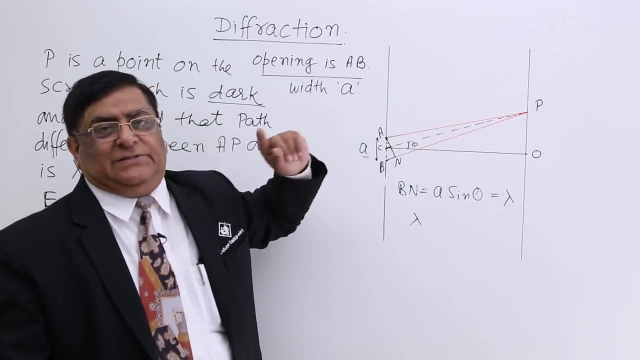 That is lambda by 2.. And if it is lambda by 2, what will be the result? Answer: result will be destructive superposition and there will be darkness. Now see another thing: From A to B, there are many sources. 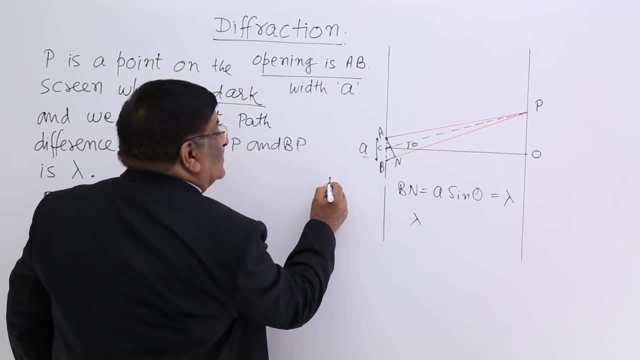 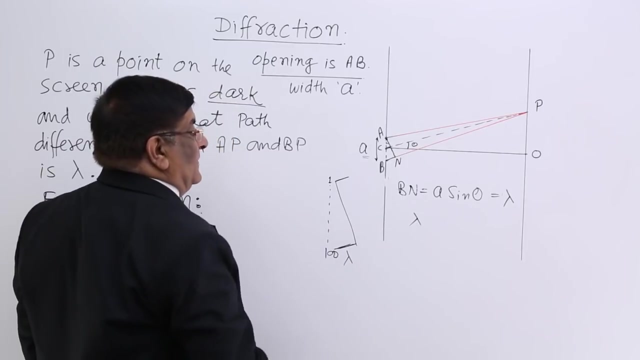 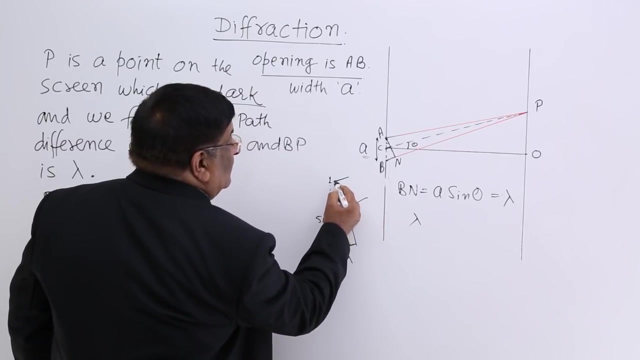 I divide these sources as source number 1 to source number 2.. How much is the path difference between wave from 1 and wave from 100?? I say it is lambda. Then 1 to 51, this: How much is the path difference between wave from 1 and wave from 51?? 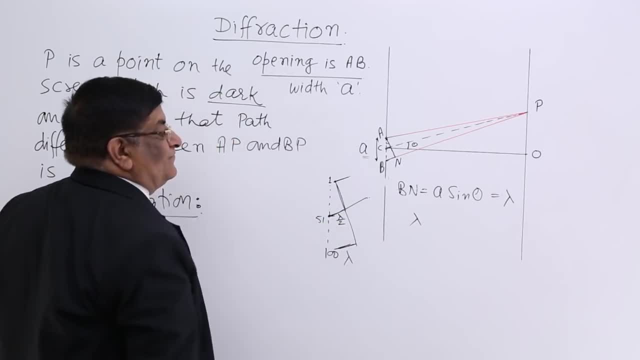 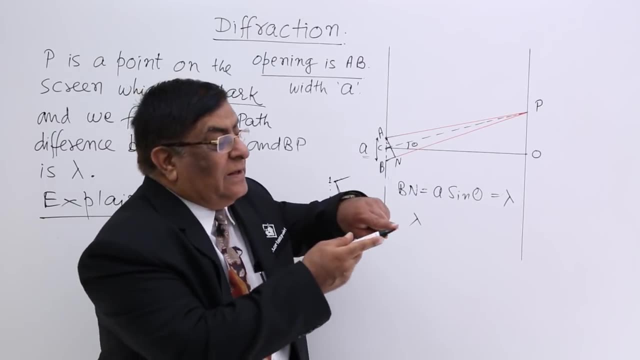 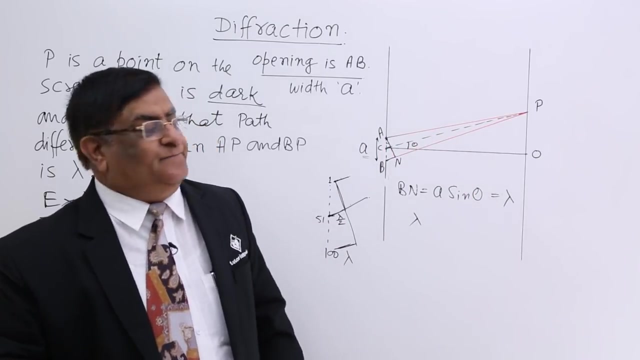 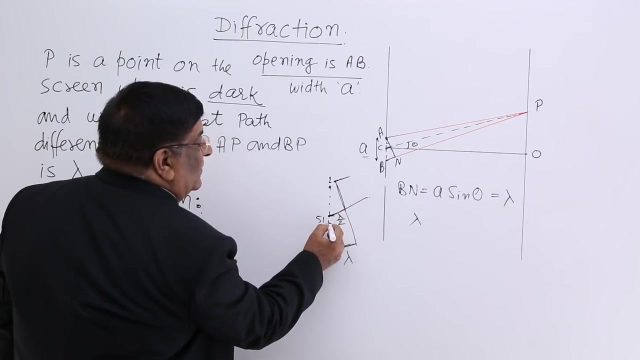 Answer: this will be lambda by 2.. So these two waves, at least according to the principle of superposition, will cancel out each other's amplitude and the resultant will be 0.. Now I take wave from source number 2 and source number 52.. 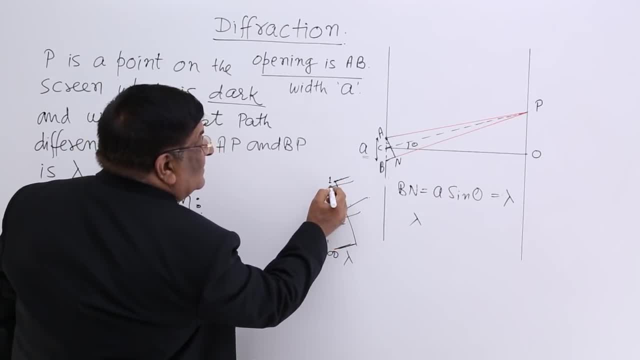 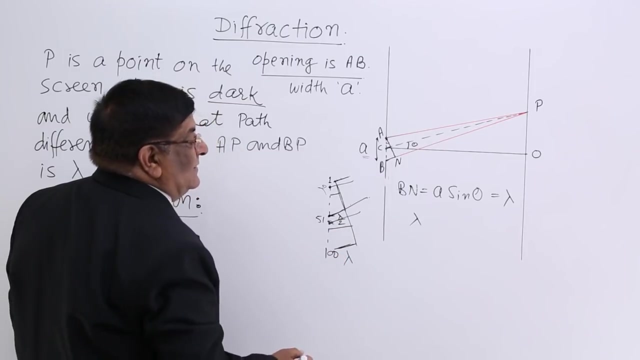 This and this. How much is the path difference? If 1 to 51 is lambda by 2, then 2 to 52, again the difference will be lambda by 2.. If I take wave number 10 and wave number 60, the path difference will be lambda by 2.. 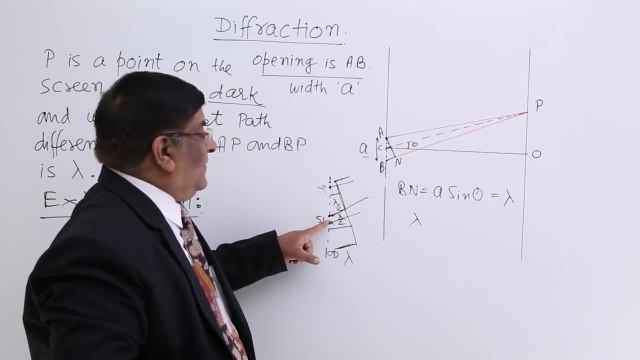 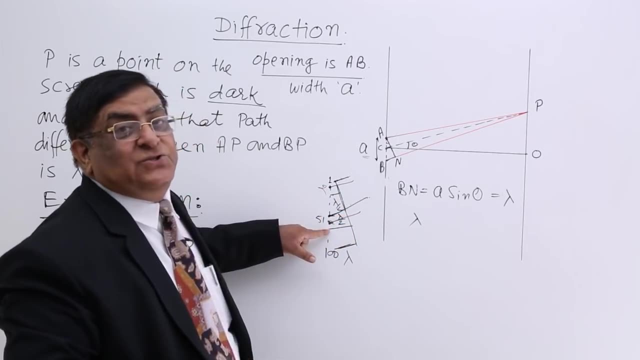 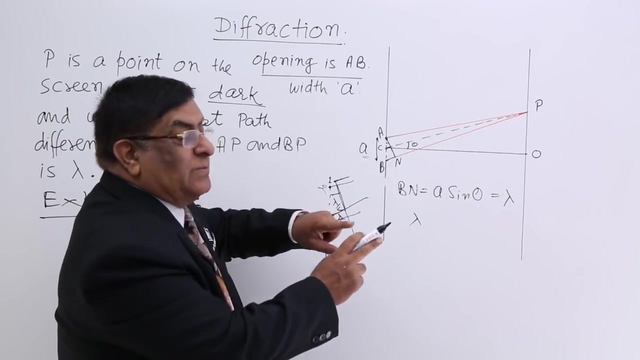 So I make pair First 51, that pair path difference lambda by 2.. 10th source: 60th source: path difference lambda by 2.. 30,, 80,, two waves: how much is path difference lambda by 2?? 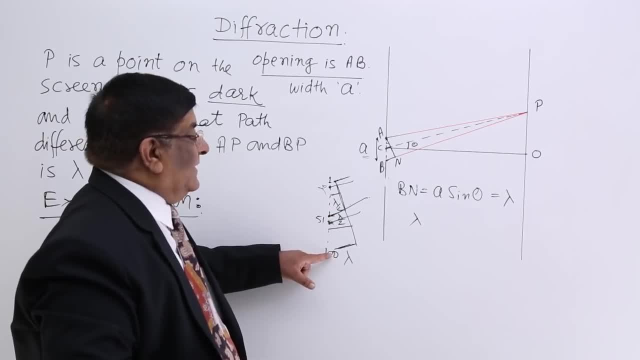 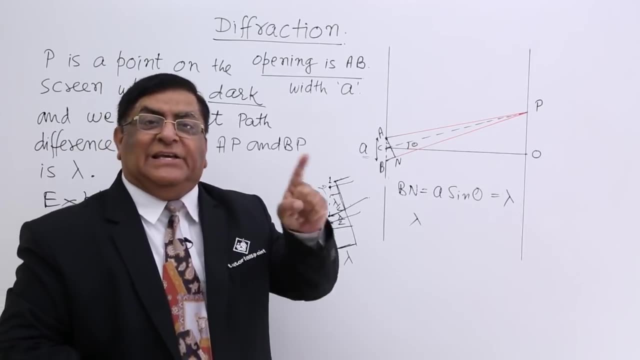 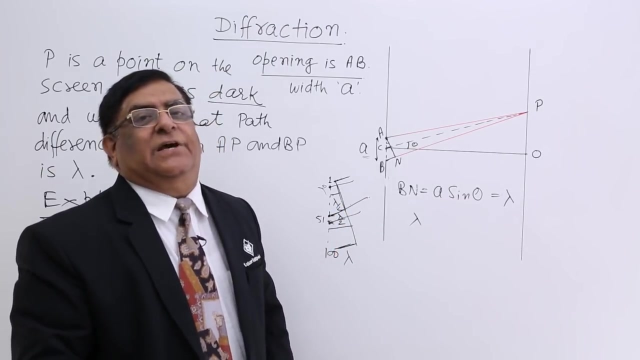 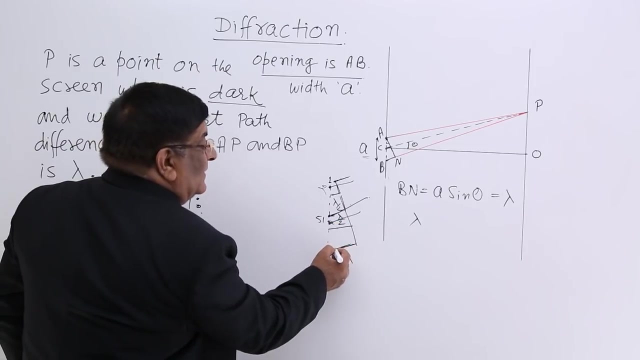 50, 100, path difference lambda by 2.. So I have got 50 pairs and each pair has got a path difference lambda by 2.. Do I have pairs which have got path difference lambda? No, Because from 1 to 100, the path difference is almost lambda. 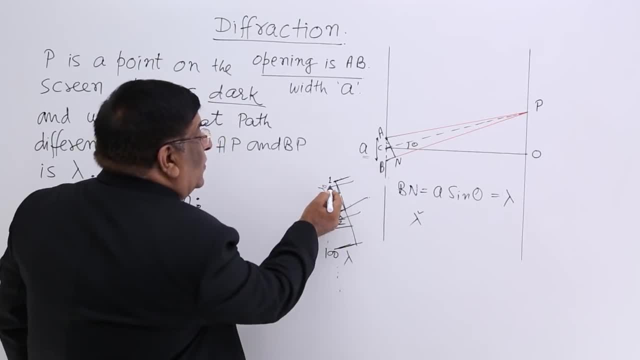 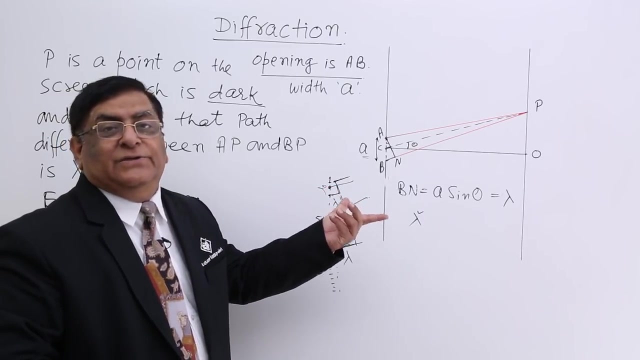 For point number 2, there is no source here, So it has no corresponding point for which the path difference is lambda. Point number 10, there is no source here which has path difference equal to lambda. So for lambda by 2, we have got all the pairs. 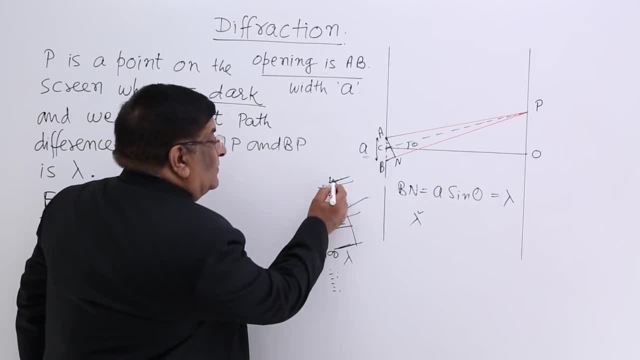 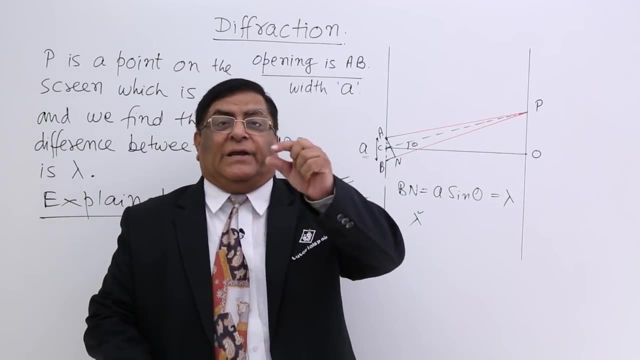 But for 1 lambda we have no pairs, Because from this point to this point the maximum path difference is lambda. So in between we have so many lambda by 2, lambda by 2.. So result of superposition for each pair. 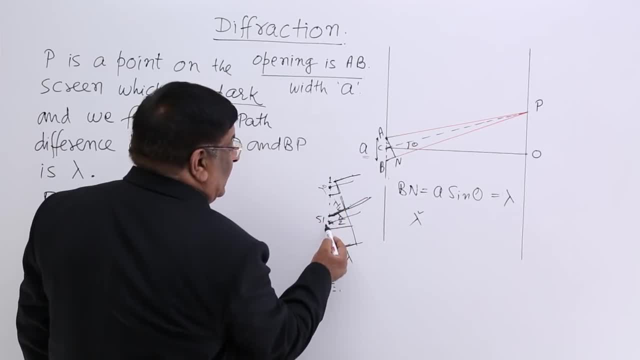 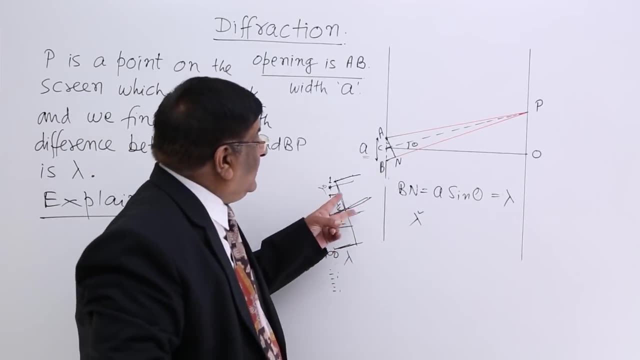 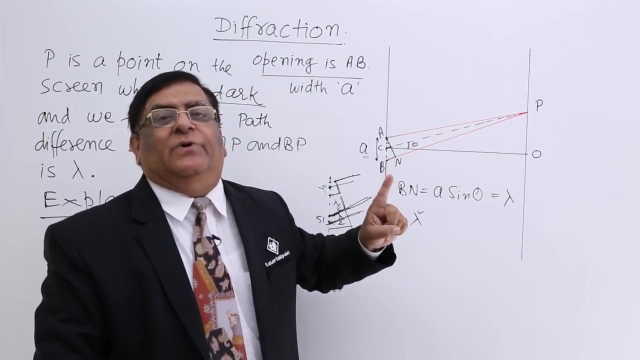 These two pairs lambda by 2, dark, These two pair, dark, dark, dark. So we get all the pairs making the point P as dark point and we do not get any pairs which will make it a bright point. So how will be the point P? 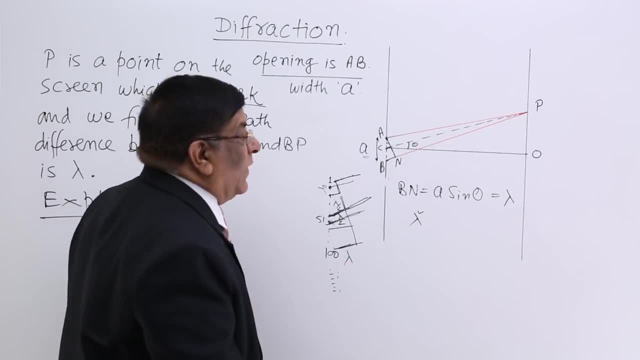 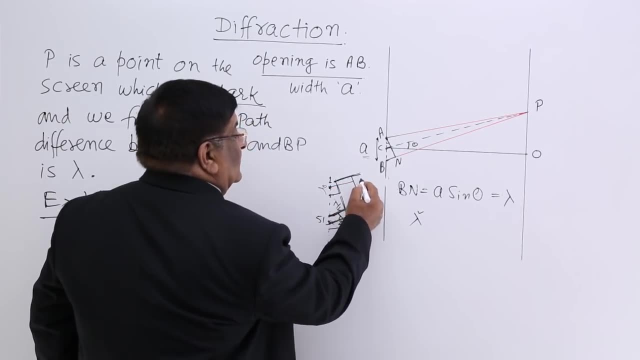 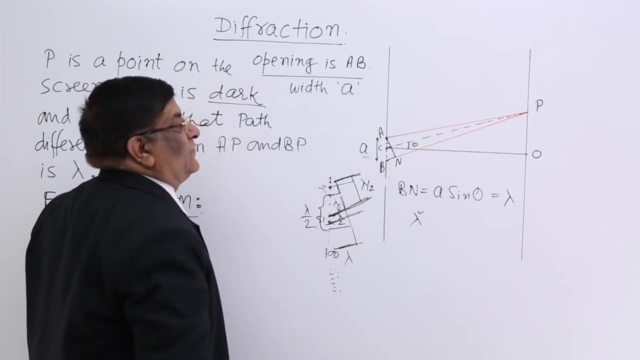 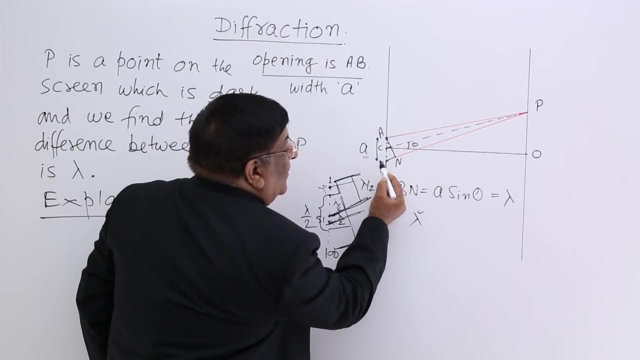 Answer is: it is a dark point. So why dark point? Because the superposition is between the two waves which have got path difference: lambda by 2.. Here, lambda by 2.. So there is no superposition of lambda, Only this and this. any wave from here, they have got a path difference: lambda. 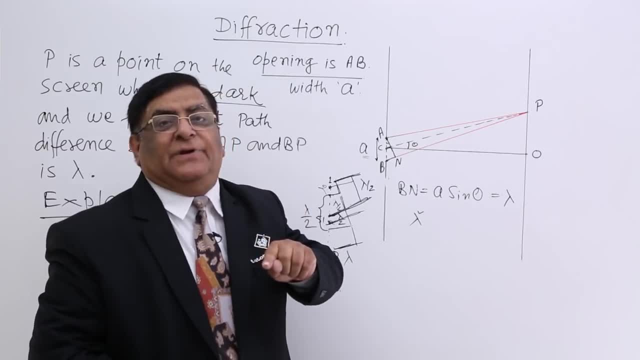 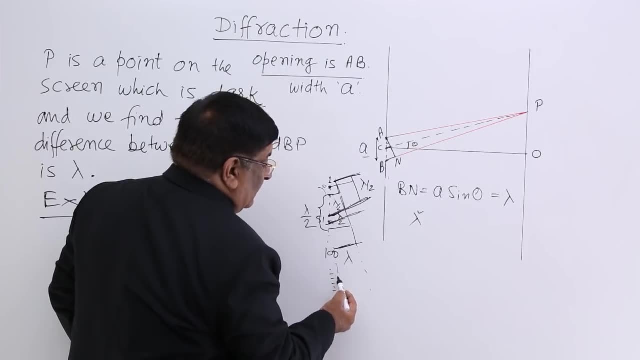 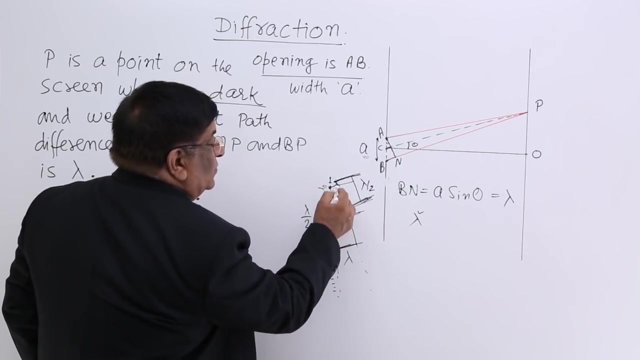 But for superposition all the waves should have path difference. lambda, There are no other waves here. There are no other waves here, So no other waves here. So they make a group like this: Superposition of this two, this two, this two and this two. 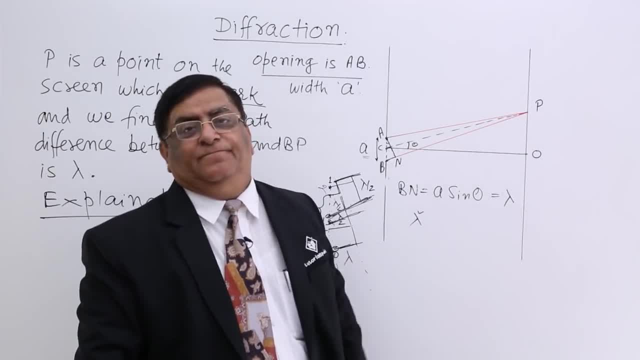 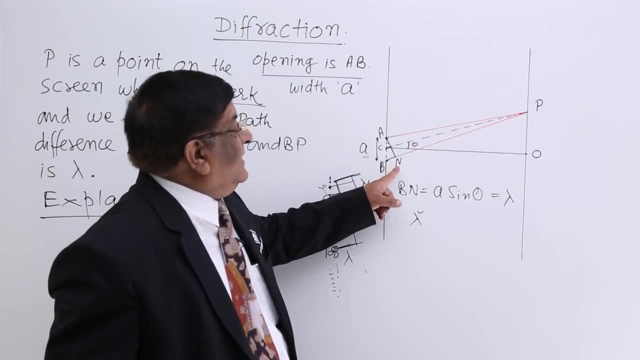 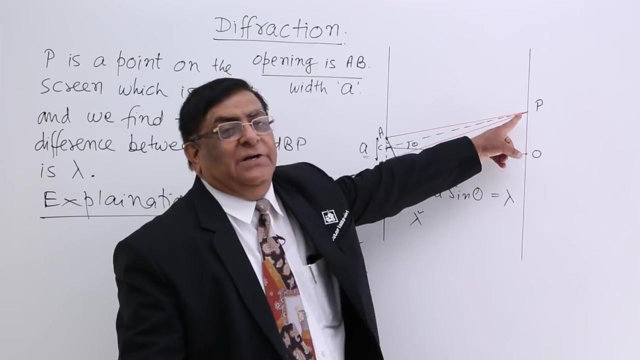 And all these pairs lambda by 2, they make it a dark point. This is explanation that why, if this path difference from A to B is lambda and we get the point P as a dark point, So this is explanation for P being the dark point. 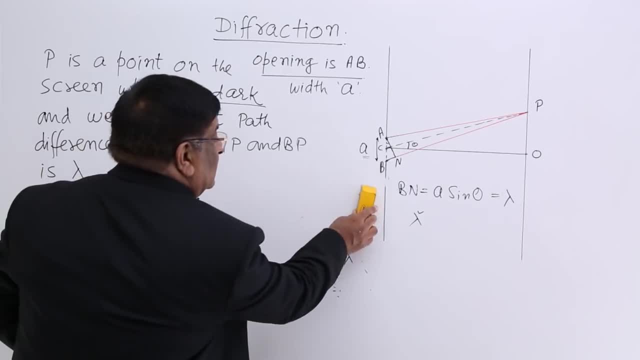 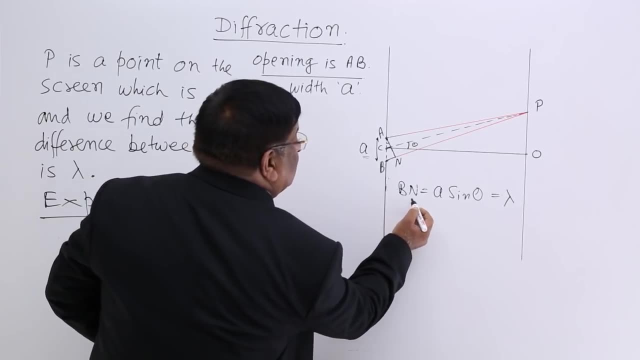 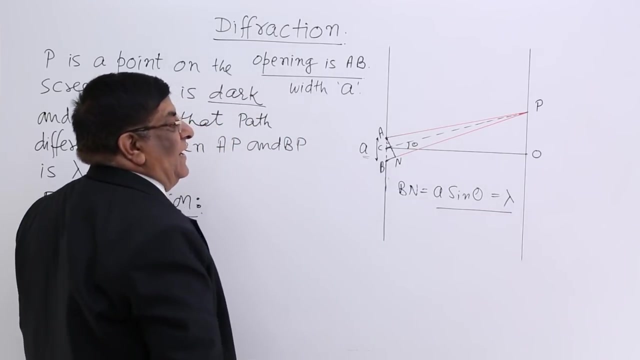 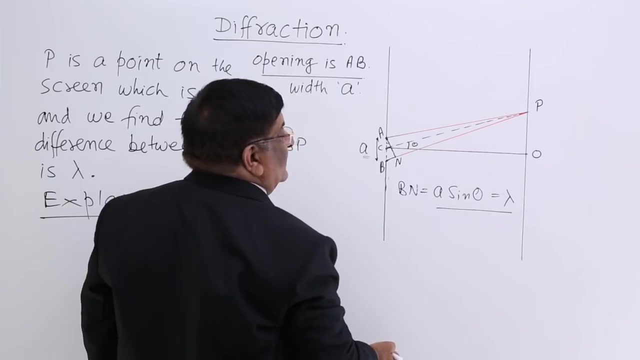 Similarly now, because this path difference, lambda, has created a dark point at P and this path difference is equal to A sine theta. we have this equation: A sine theta is equal to lambda. This is the condition for dark point, This elevation theta for the first dark point. how much it is. 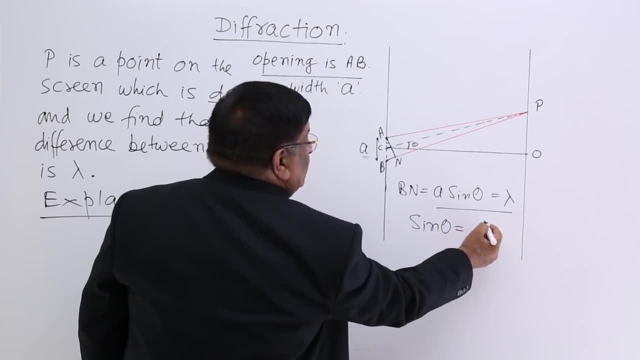 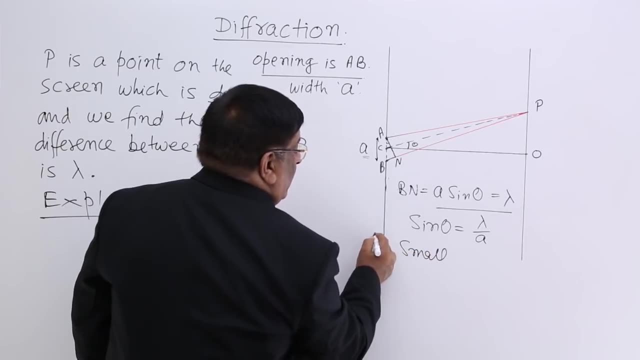 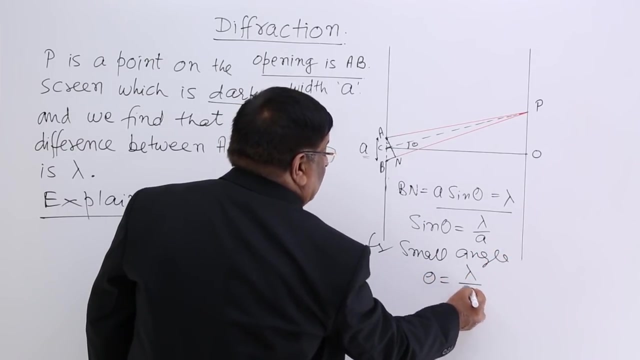 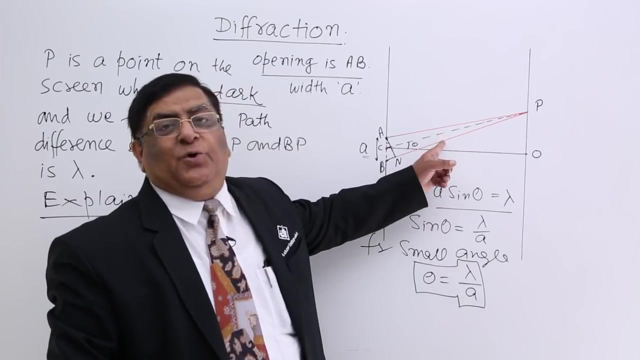 Answer: sine theta is equal to lambda upon A For a very small angle. for small angle, theta is equal to lambda upon A. This is the essence of diffraction. What is theta? It is very important. angle. Here is an opening. 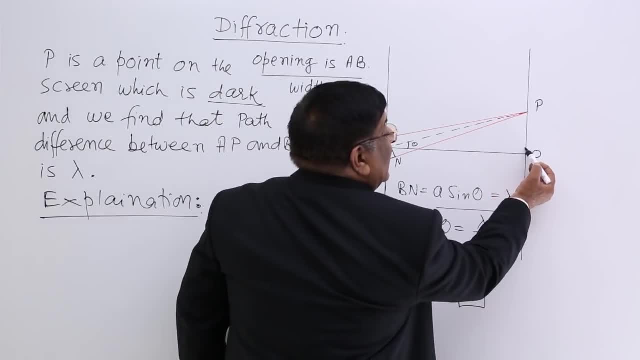 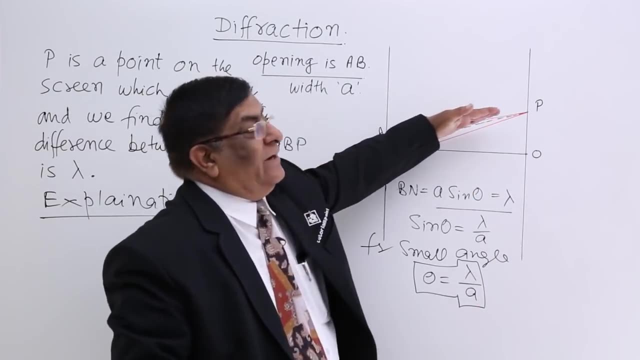 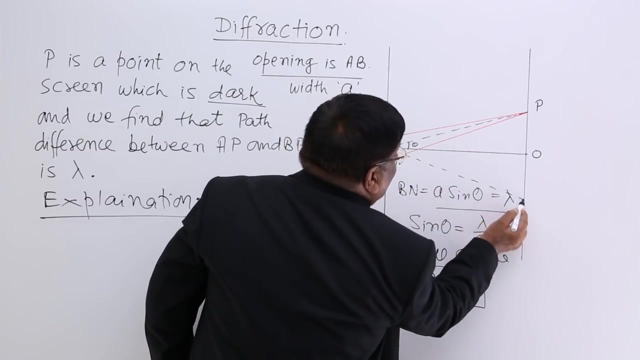 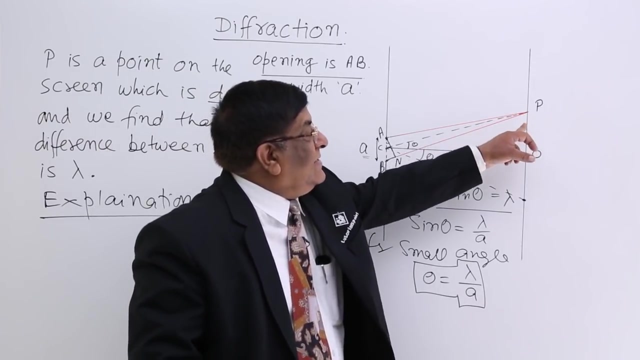 The light goes here, We get it bright, bright, bright, bright, bright. first dark. And the first dark is at what angle? Theta. Then the first dark on this side will also be at angle theta, Theta. So this is the area where there is no dark point. 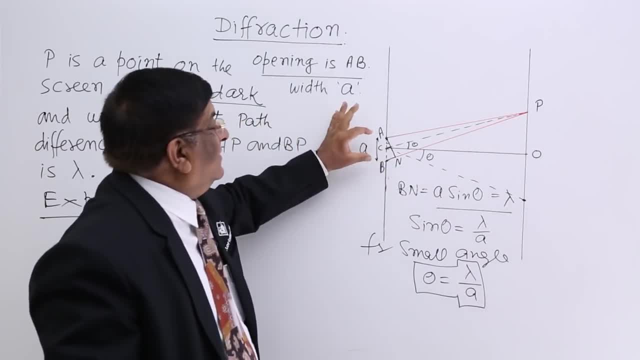 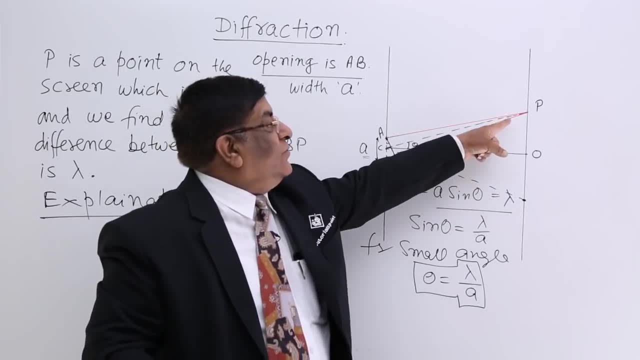 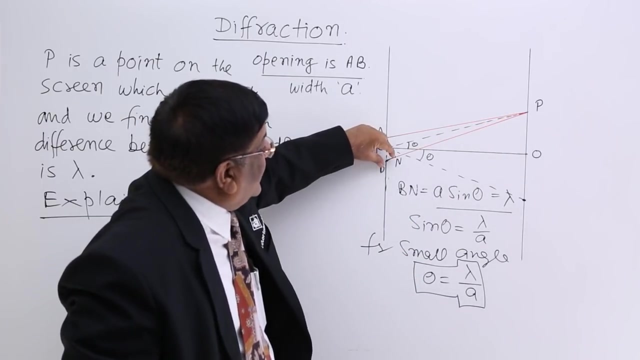 This is the total bright area and this opening is larger than this opening. That means light has been This way. there is no dark point here. This is the first dark, This is the first dark, And this first dark will be there when this path difference is lambda. 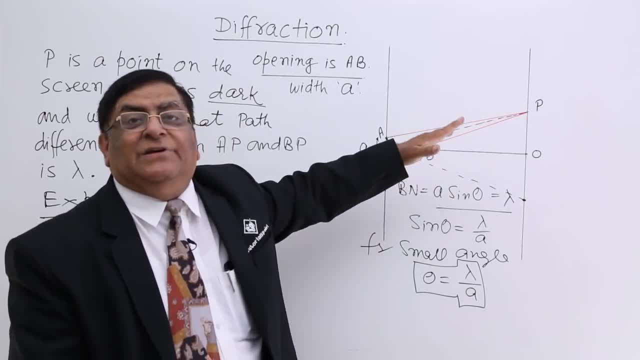 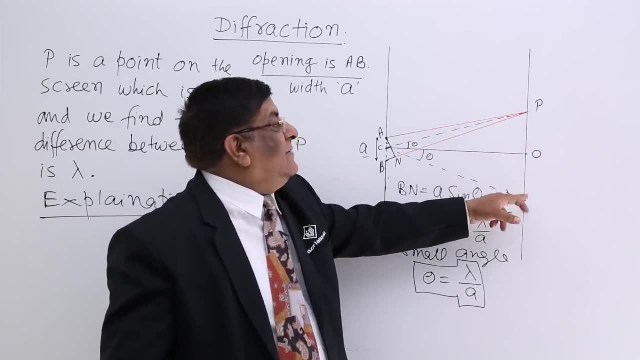 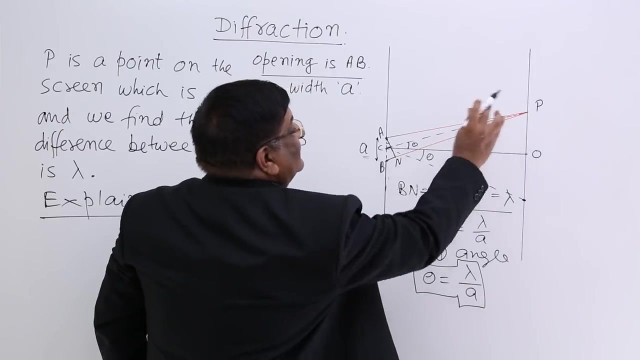 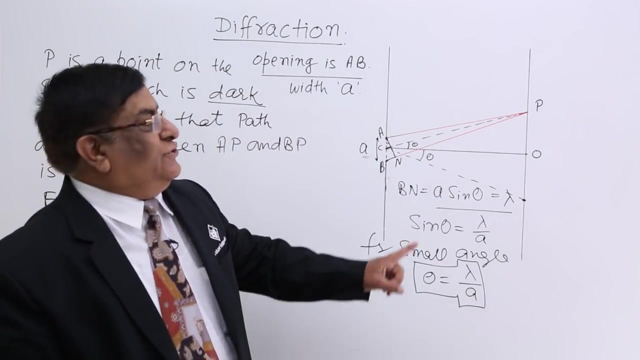 and there is the elevation of theta. So any elevation will make this opening a larger opening. So this is a larger opening and here it is a proof that light has been by these two lines. So that is why this central maxima has become a larger portion. 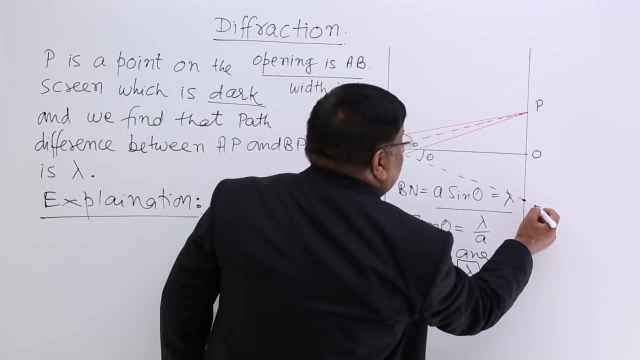 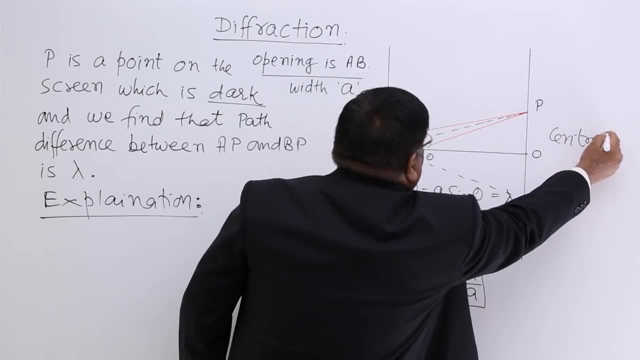 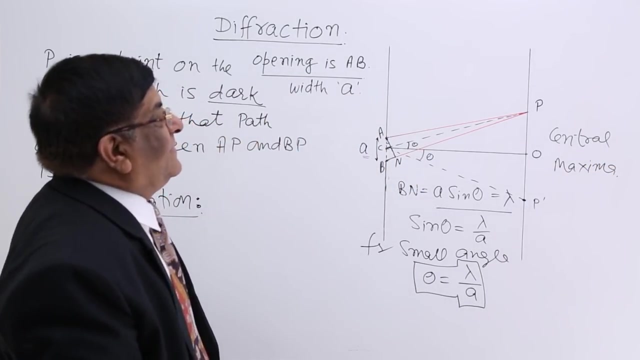 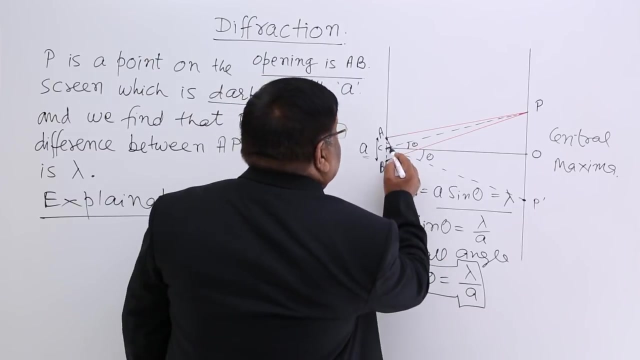 So this is the first dark here and this is the first dark at the bottom, And this we call central maxima. If we want to find out what is the measurement with respect to A, We can always find it out, And that is, if this distance is equal to D. 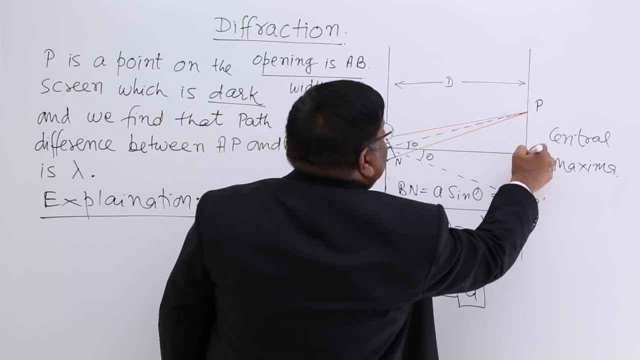 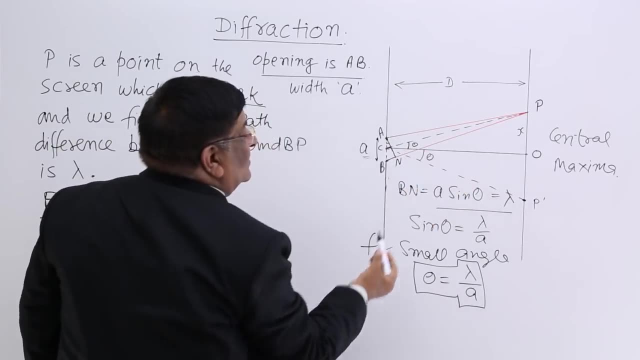 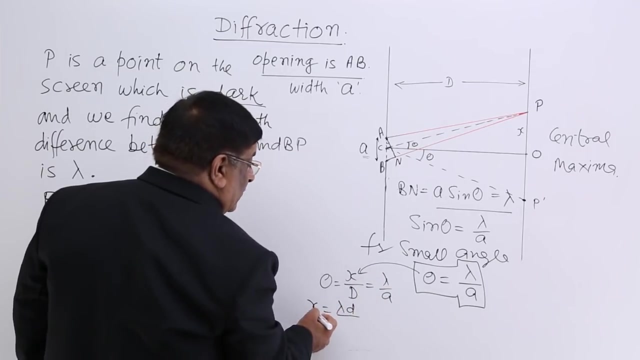 This distance And this height is equal to x, Then x upon D is equal to theta, So theta is equal to x upon capital. D is equal to lambda upon A, So x is equal to lambda D by A. This is very similar to interference fringe. that was lambda D by D. 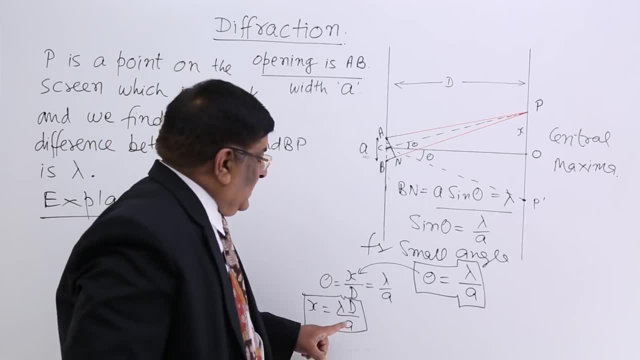 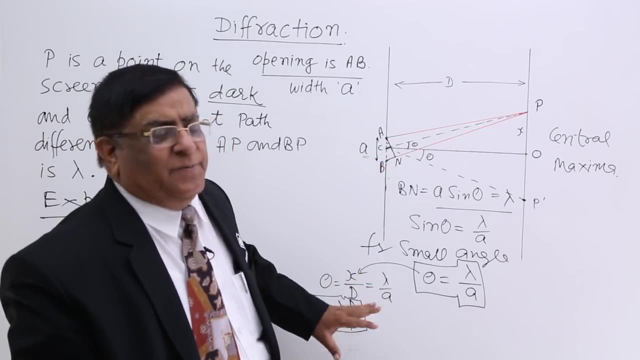 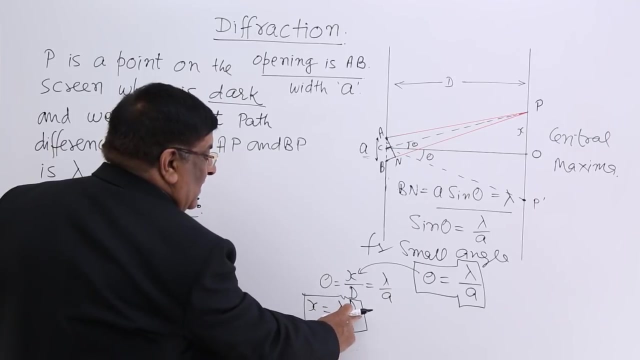 And what was that small d? The distance between two slits. and here, what is A? A is this opening, that is, distance between first and the last source. So they are similar to each other this way. Now this x width depends upon lambda D and A. 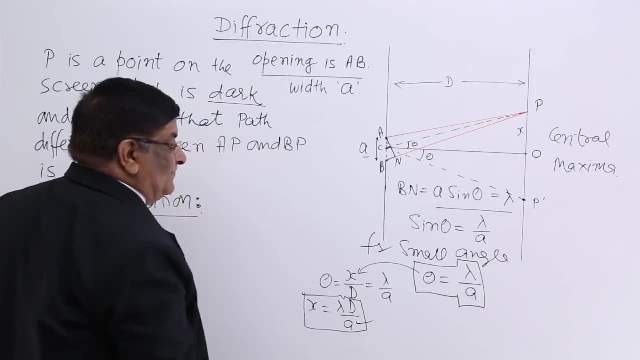 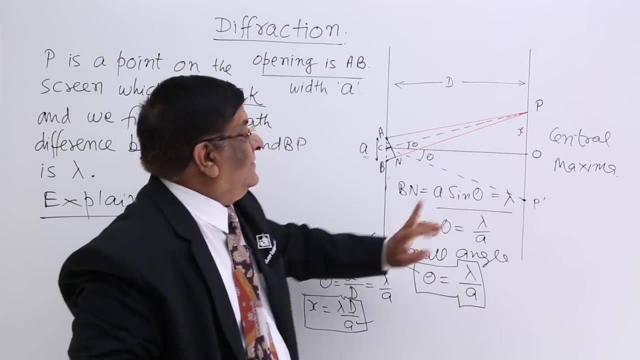 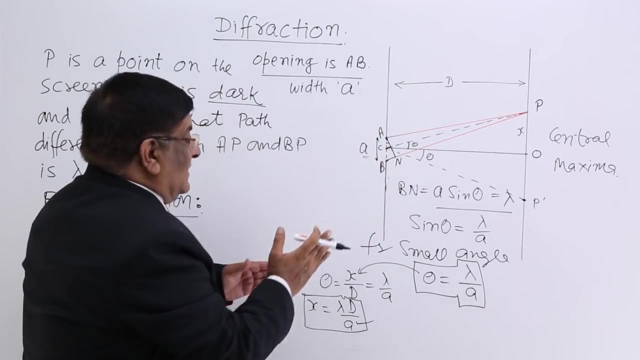 Basically it depends upon A: Smaller is the A, wider is the area this area See. So if this opening is smaller, the angle will be larger. If this opening is smaller, the angle will be larger. That is one. 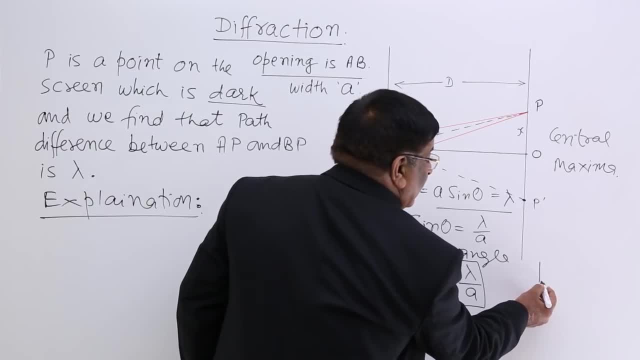 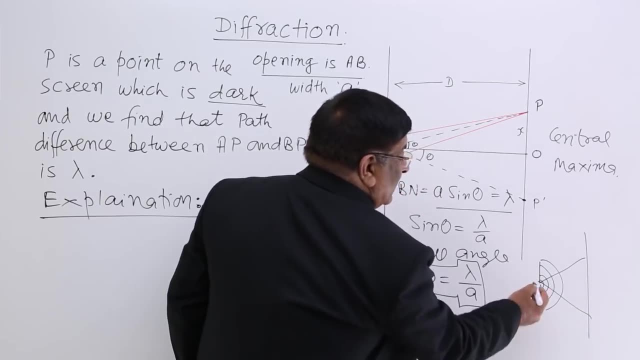 Remember. So if we have a very small opening, then it will be like this, And we get this theta. But if this becomes larger, then what do we get? We get it like this, And it is this way: smaller one. 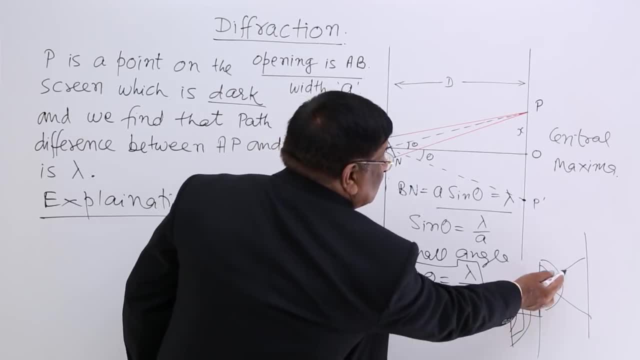 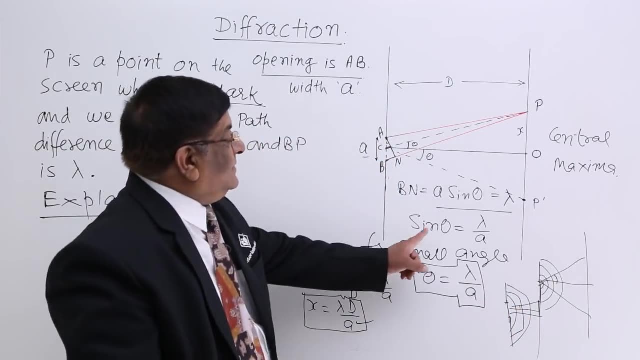 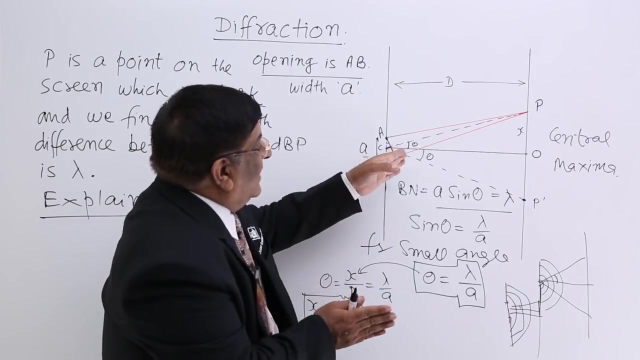 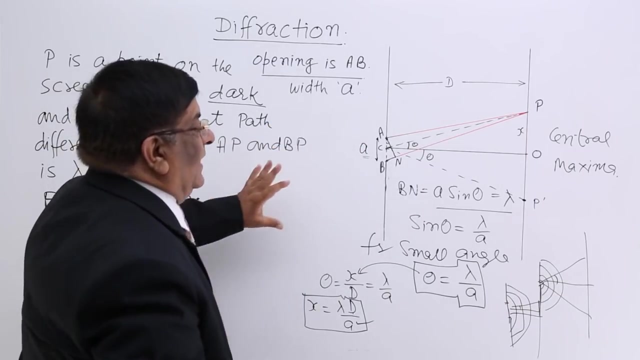 Larger than this, of course, but this angle will be. this angle will be small If this opening is wide, because this is our formula, lambda upon A. So for smaller the angular diffraction will be more. Remember this. So this is the first dark point in diffraction.